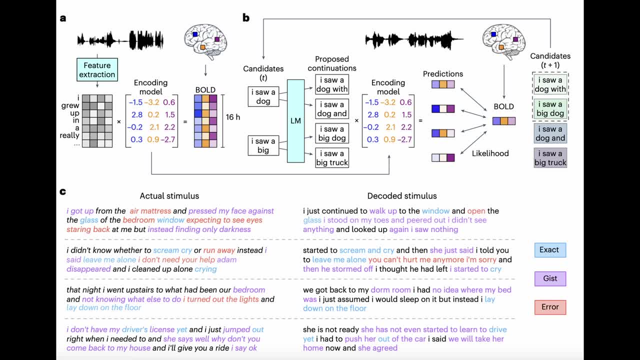 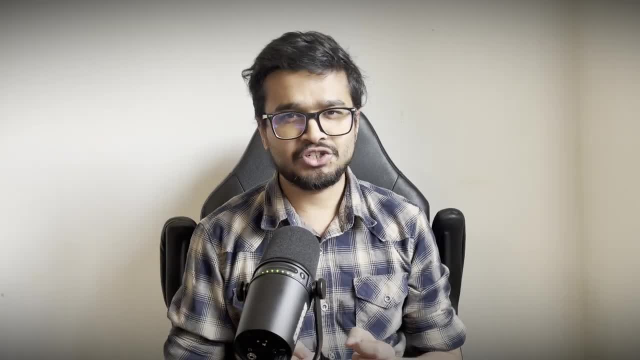 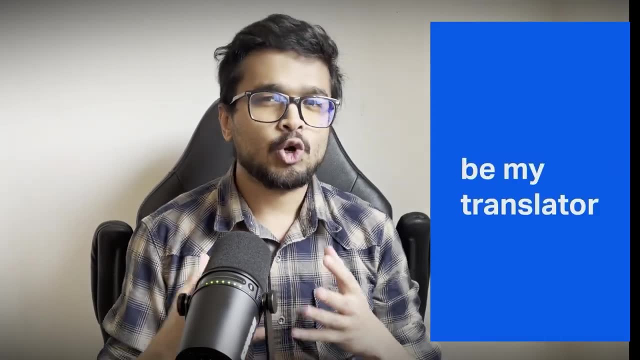 a GPT model to predict what the humans are thinking in natural language, given the auditory input that they perceive, and showed that the AI can guess what the human is thinking about 50% of the time. Another work is this: Be My Eye technology that uses GPT-4 to assist individuals with blindness or low vision to provide auditory 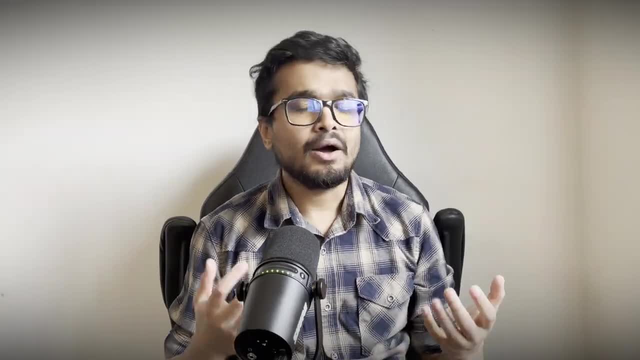 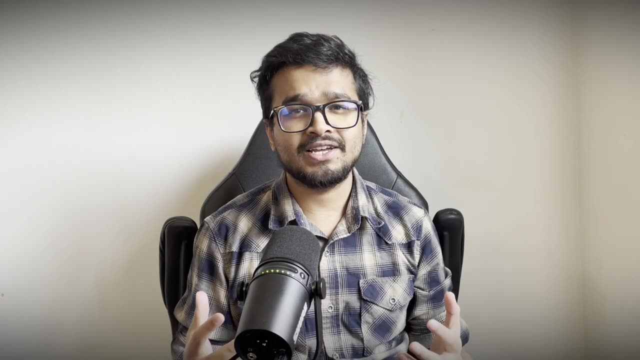 feedback describing the world around them. As you can see, multimodal learning is a fast growing space of AI research and, in my opinion, the next big milestone that's going to bring the next leap in intelligence is going to come from this area. Note that this video is not going to 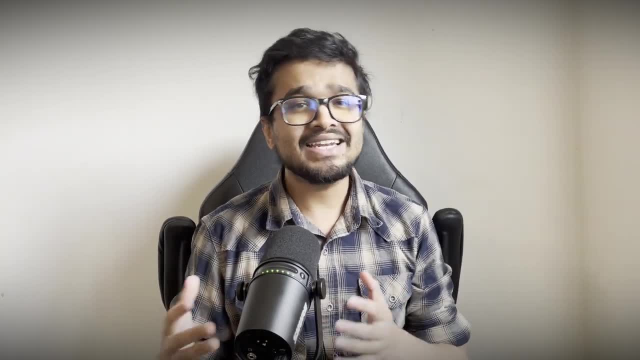 cover generative image or text-to-image models like DALL-E or Stable Diffusion. That deserves its own video, and I plan to do one in the near future. So until then, thanks for watching and I'll see you in the next video. 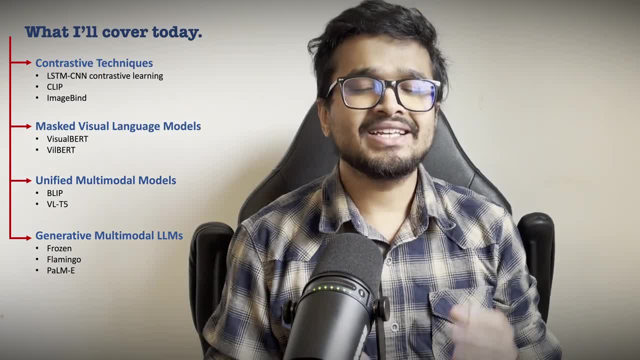 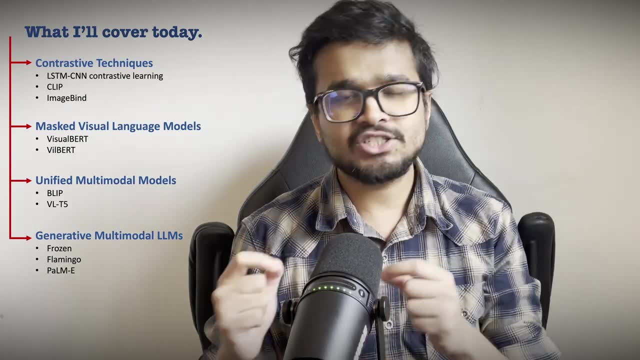 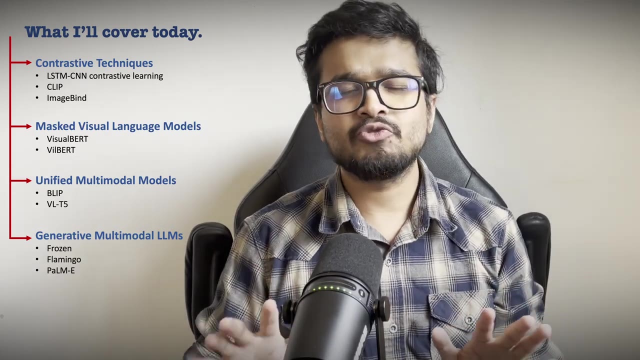 Instead, this video will cover the key ideas behind training neural networks that can learn from multimodal inputs, and the basic concepts and solutions in this evolving field. Concretely, I'm going to go over 10 important research papers over the last few years that will broadly cover. 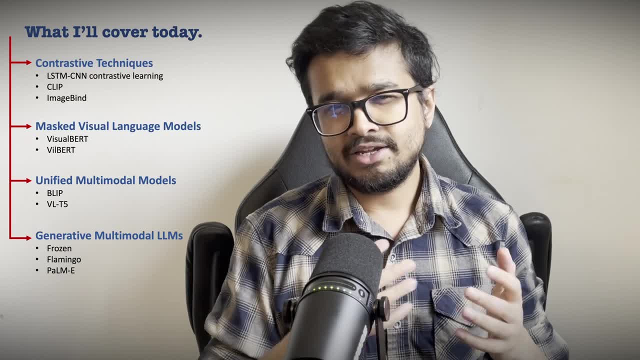 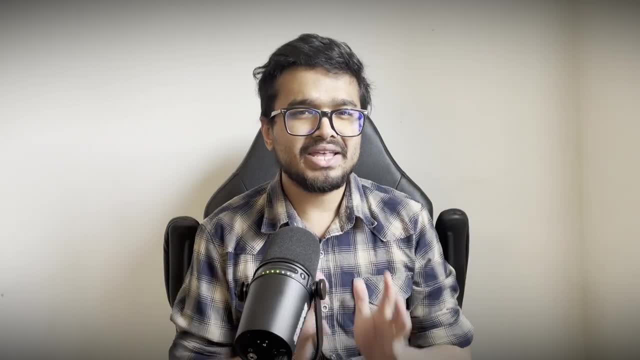 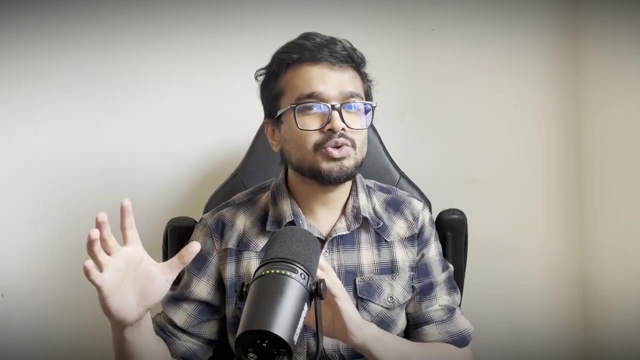 most of the different approaches in the field, their advantages and disadvantages and the many innovations they have brought over the last few years. I've deliberately picked methods that use images and text, because I think those are the easiest architectures to develop the most intuitive understanding of the topic, If you like this. 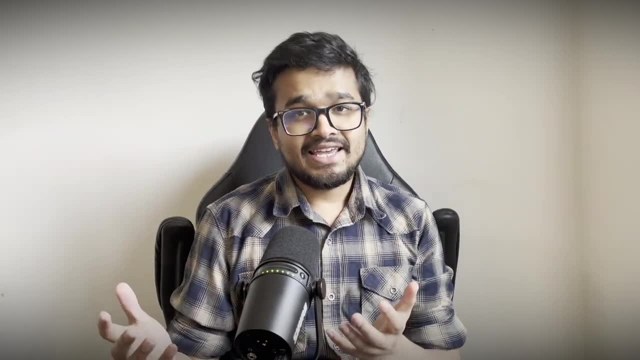 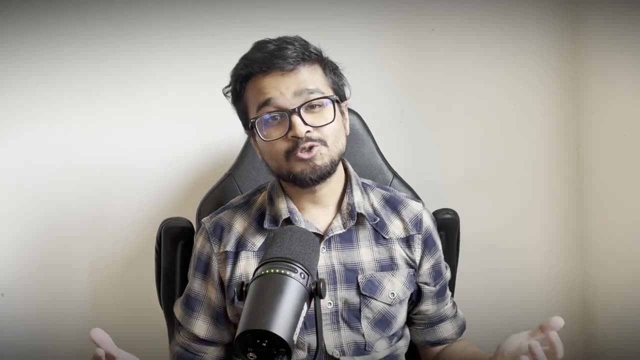 video and the content I'm producing on this channel, like the AI breakdowns and the AI devlogs. please consider subscribing. Your time, interactions, feedback mean a lot to me. You are all magnificent, So, without further ado, let's begin this new episode of Neural Breakdown. 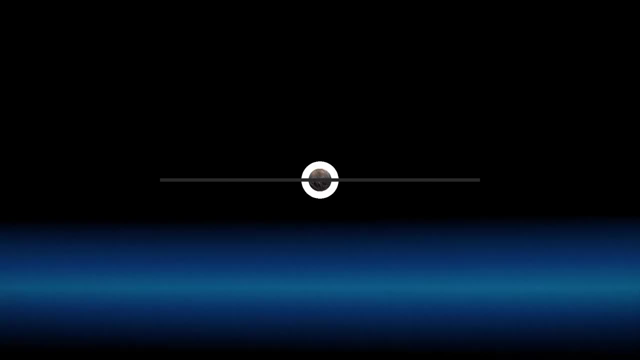 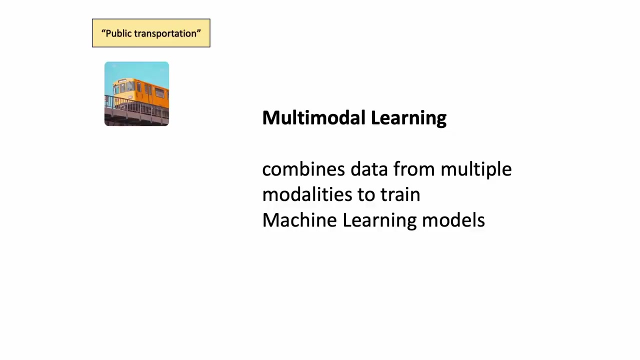 Nothing But Neural DefiniiNals. In multimodal settings, the input data can include information from multiple modalities, such as text, images, audio video, heat maps, 3D, volumetric data, anything. The goal of multimodal modelling is to learn the dependencies and relationships between. 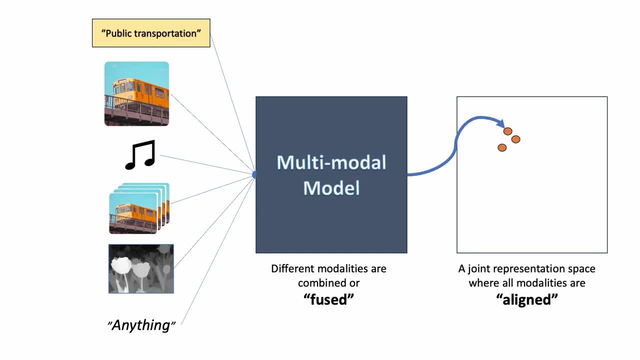 these different input types and then align each of them to a joint representation space where these different modalities can follow. Like we saw in the first video, the different input models use on a specific region every time and create interdependent combinations to freely Communications for varうわise. 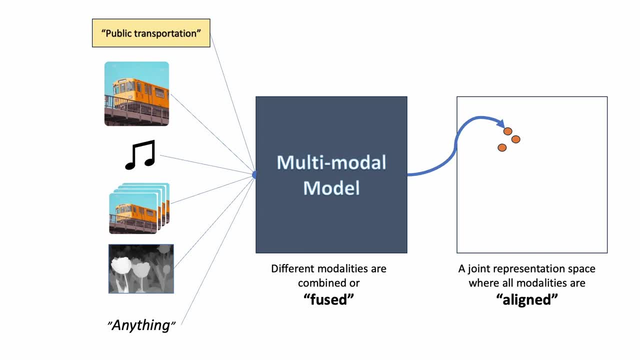 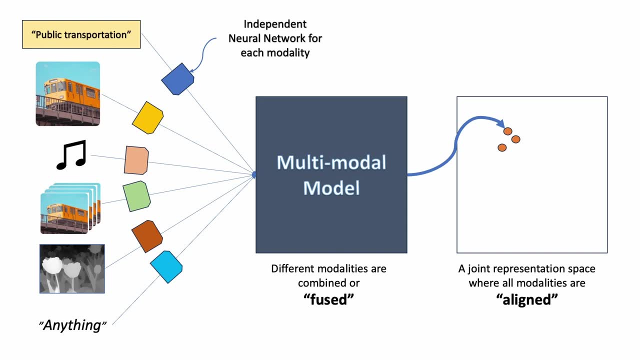 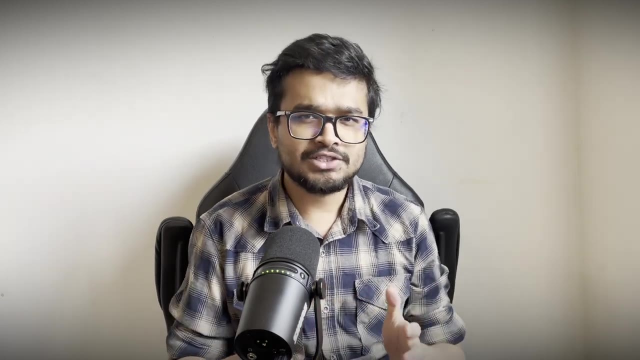 effectively interact, enhance and complement each other. A common first step is to independently embed each of the input modalities through their own appropriate neural network to form these unimodal embeddings. This means that we can choose to use an RNN or a transformer to embed a sentence as a. 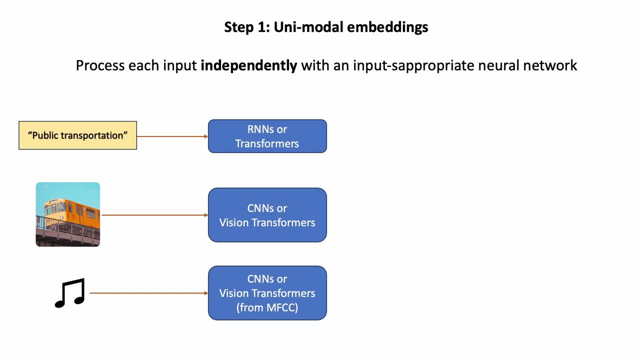 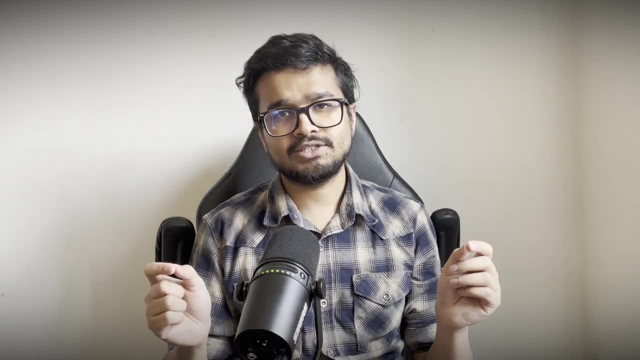 sequence of tokens and a CNN or a vision transformer to embed an image or the MEL spectrogram of an input audio sample. Following this, we have a fusion step that fuses these unimodal embeddings into a new joint representation space that allows for cross-modal interactions. 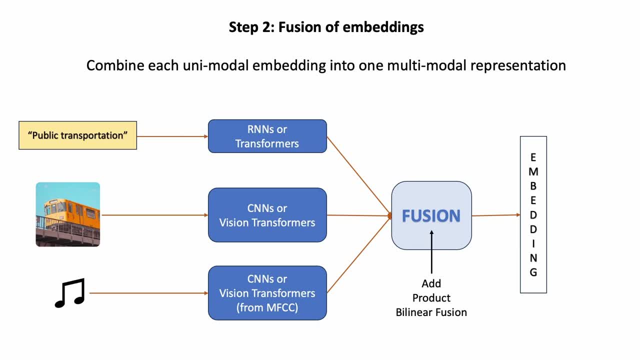 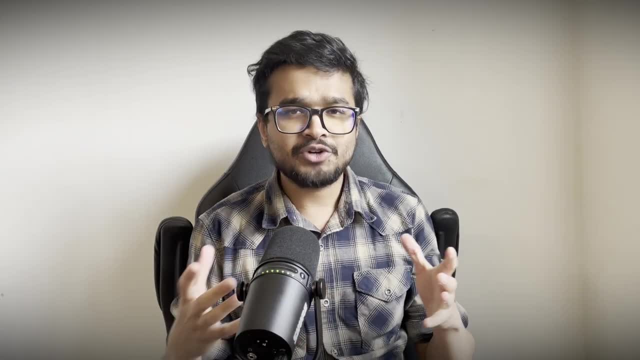 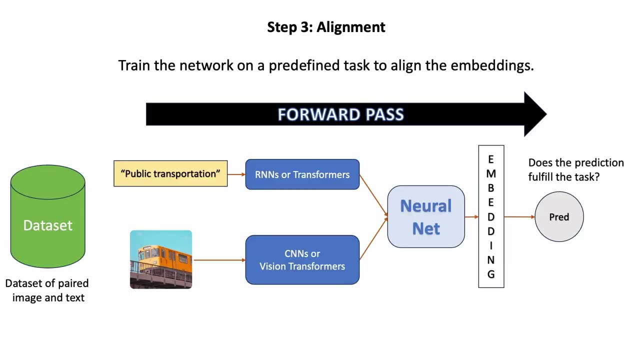 These fusions could be additive, multiplicative concatenation, an outer product or, most commonly, another neural network. After fusing the two representations, we train the neural network, on a predefined task, to align these embeddings via backpropagation. In other words, we take a dataset. 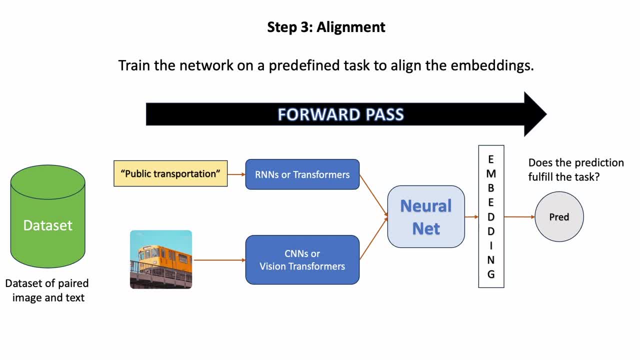 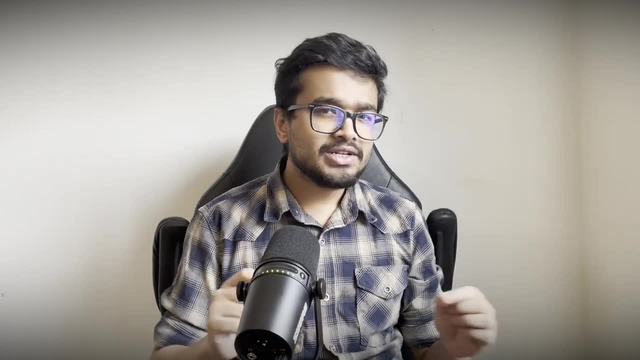 We forward, pass the data through the network to receive an output, we calculate the loss of the network's output to our target solution and then we update all the weights in the neural network to optimize the alignment of this joint embedding space. The choice of this training task often dictates what network architecture loss function. 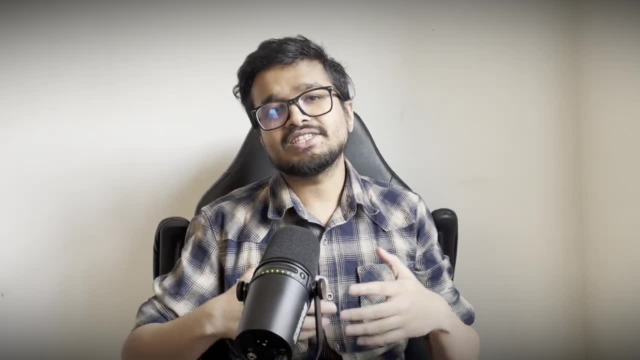 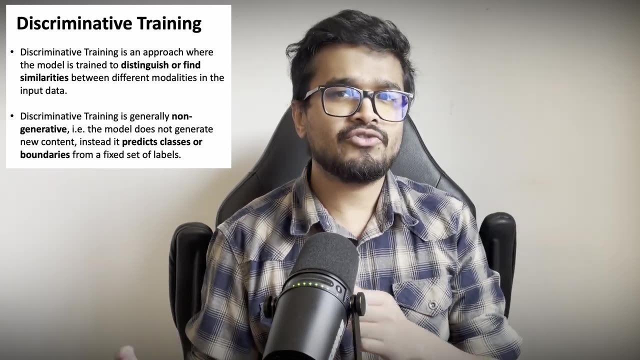 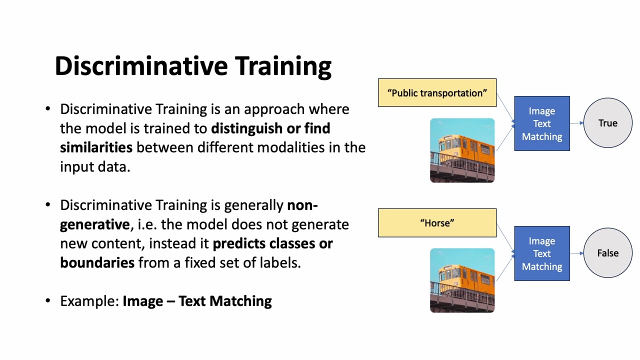 and datasets we use for training. One family of such tasks is discriminative training. Discriminative training is an approach where the model is trained to distinguish between or find similarities between the different modalities in the input data. They are often trained to learn a specific decision boundary and optimize on a single. 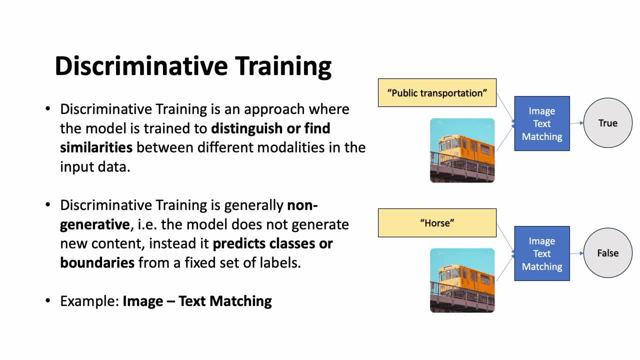 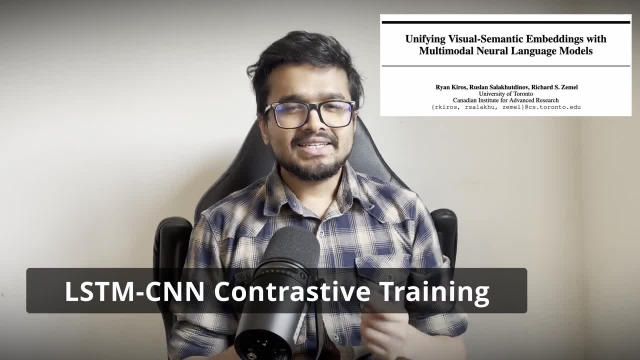 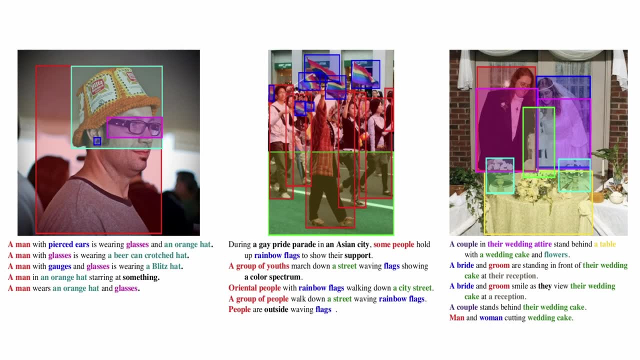 task, for example, to match captions with correct images. The earliest paper that we are going to talk about today is this amazing work from 2014, where they train the model on this image-text matching objective. The dataset is the Flickr 30K, which contains 30,000 images. 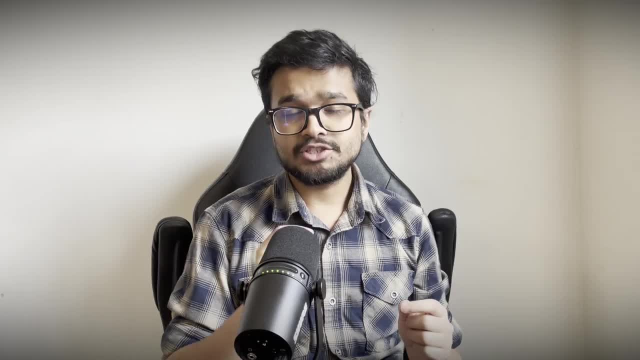 The data set is the Flickr 30K, which contains 30,000 images, and all measuring answers are the lighting versus contrastいう image 28,000 from Friday to Sunday and a FOA 18,000 instantaneous times per hour. 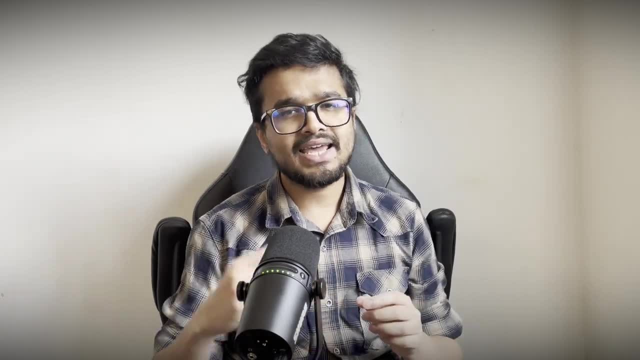 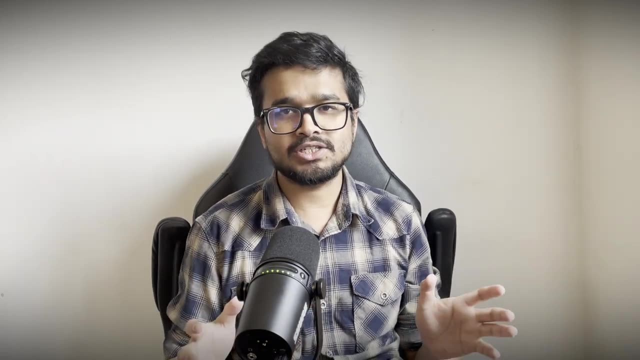 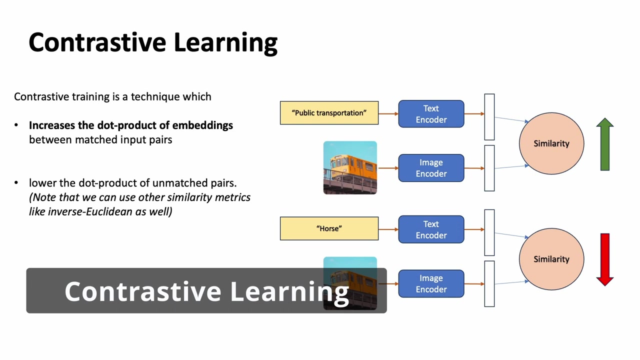 around During training. they separately process the captioned text and the paired images with CNNs to form unimodal embeddings for both sources and then use contrastive training to align them. Contrastive training increases the dot-product similarity between matched input and. 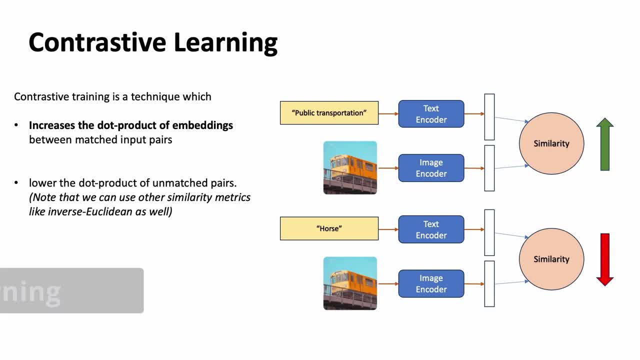 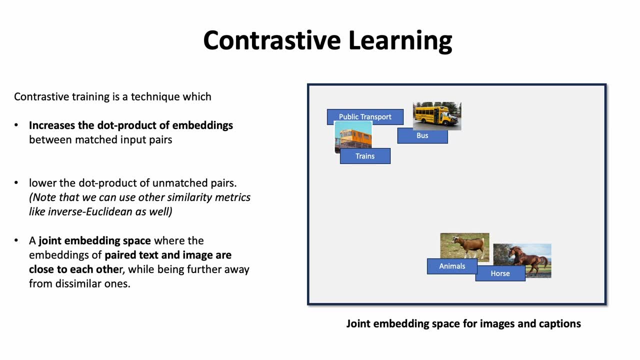 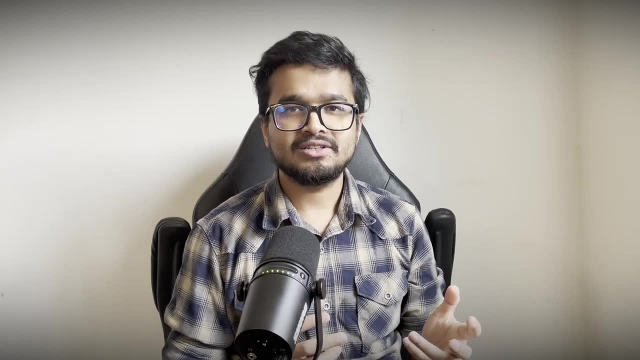 image-text embeddings. lower-input dot-product排 page of unmatched pairs. This trains a joint embedding space. the embeddings of paired text and images are close to each other while being further away from dissimilar ones. they showed some incredible results for cross-modal retrieval. for example, if you search the nearest image embedding of: 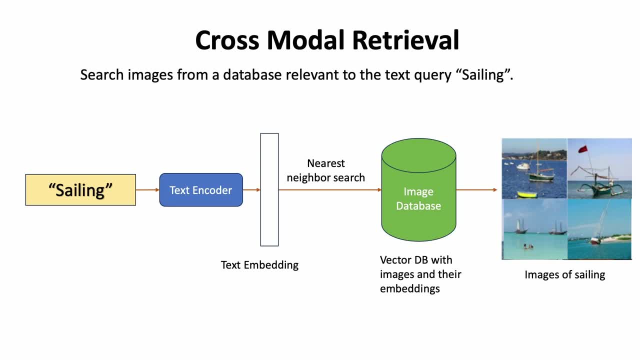 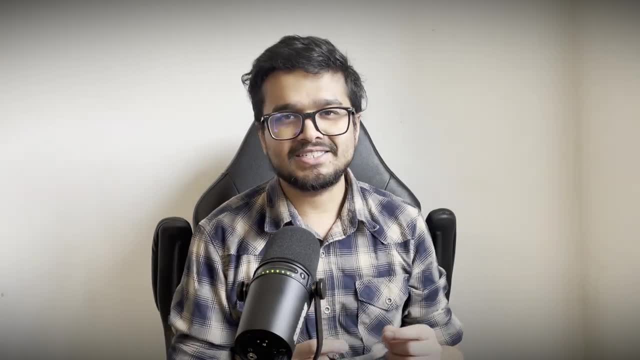 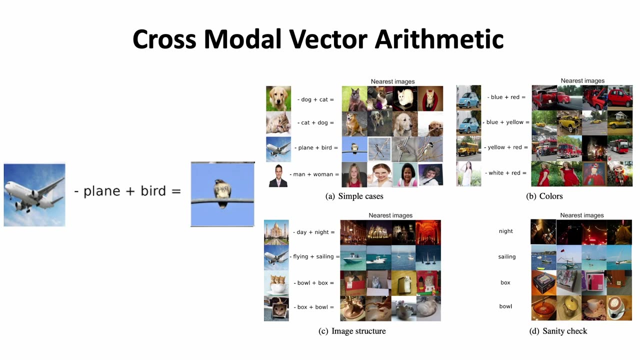 the text sailing, you're gonna get images of sailing. they also show one of the coolest results ever of doing vector arithmetic in multimodal space, where they subtract the embedding of the text plane from an image of a plane, then add the text embedding of a bird and searching for the nearest image returns. 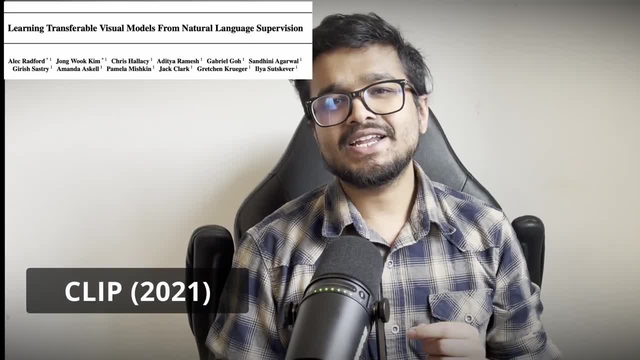 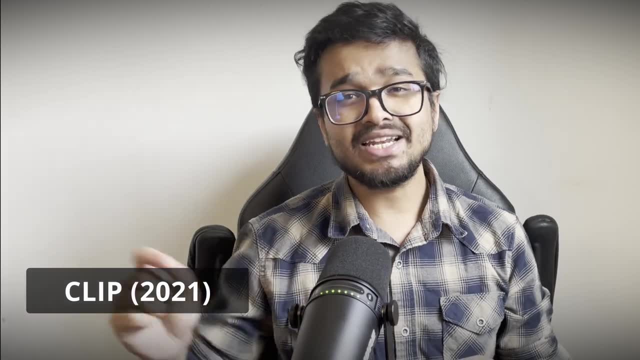 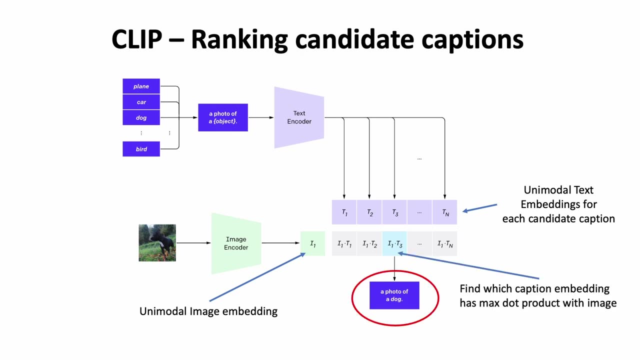 images of birds. what clip is open eyes? version of contrastive pre-training on a new data set that they created called web image text, which contains 400 million image text pairs. after training, the model can input an image and a list of candidate captions and then output a confident 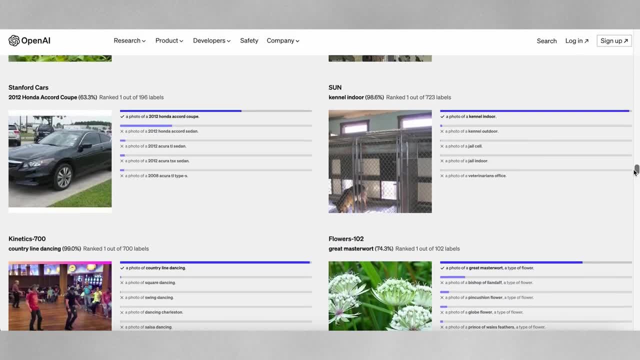 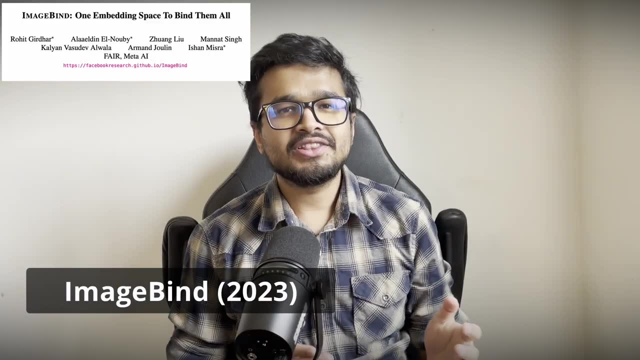 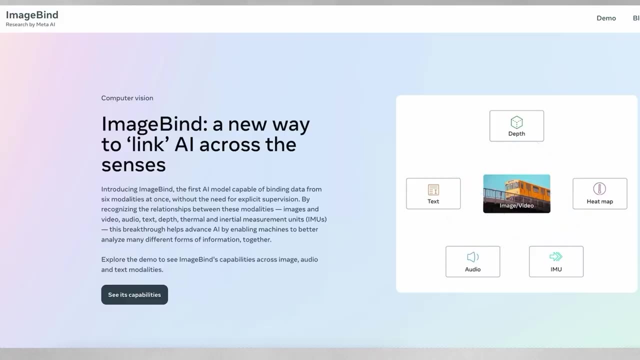 score for each of the captions. clip demonstrated zero-shot learning, meaning it could recognize objects even though it wasn't direct trained on it. pretty cool. right recently we got the image bind paper from meta, which combines multiple multimodal sources like images, audio text, depth heat maps I am use, into a single model. it is not possible to 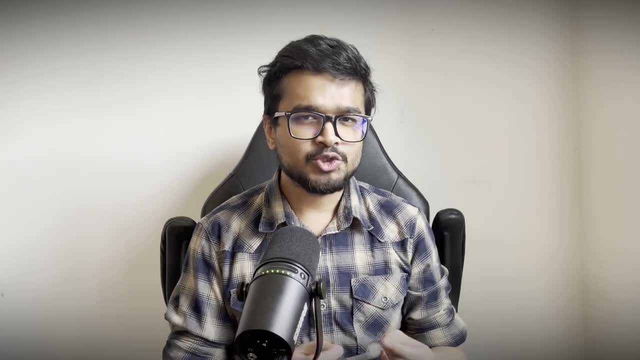 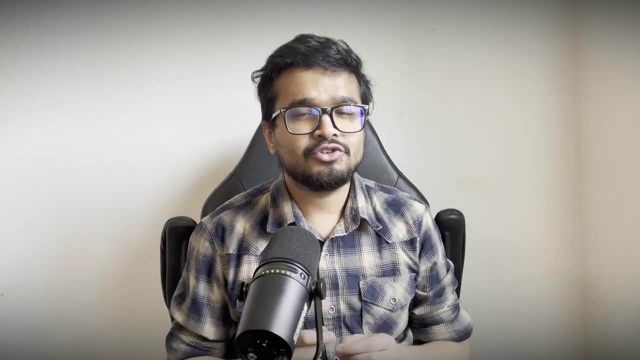 acquire a data set large enough that has matched inputs of all these input types present together. so what image bind does is to learn this single shared representation space. using contrastive learning, they train to align images with text, images with audio, images with text, images with text, images with text images. 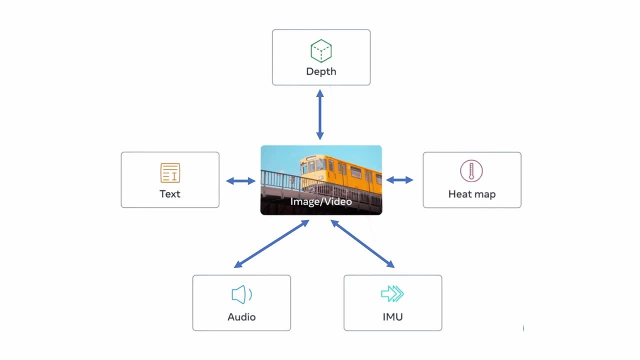 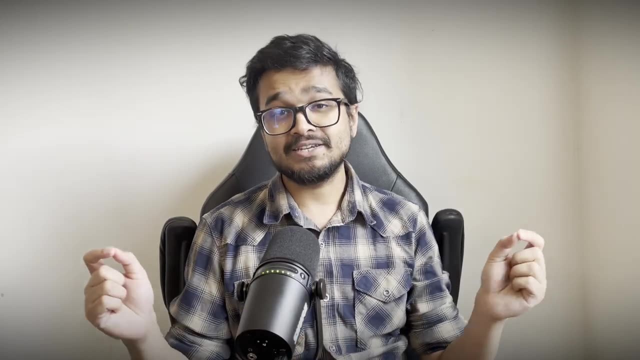 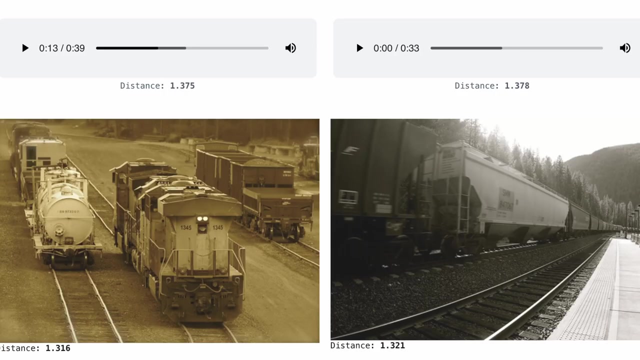 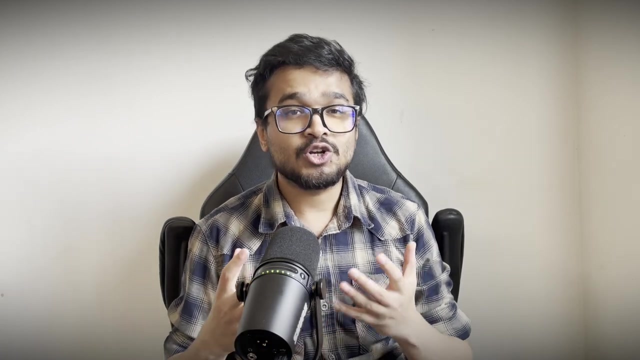 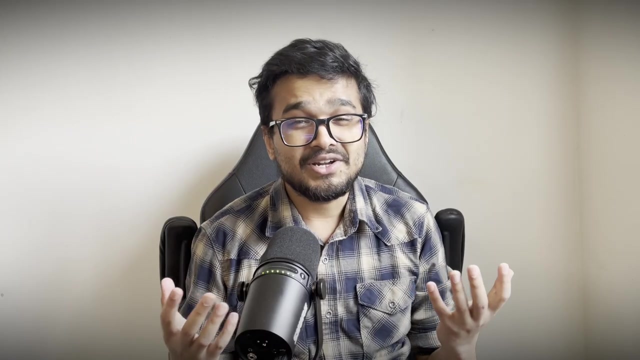 audio images with heat maps and show that by doing this on a large scale model, it is like audio and texts are also aligned. this resulting model is crazy. discuss cross model retrieval. Tim Kahlo, latin speaking on top and etpee beille reading, etc. dole sitting on a beach. that's crazy. I don't even believe all this. but so contrastive. 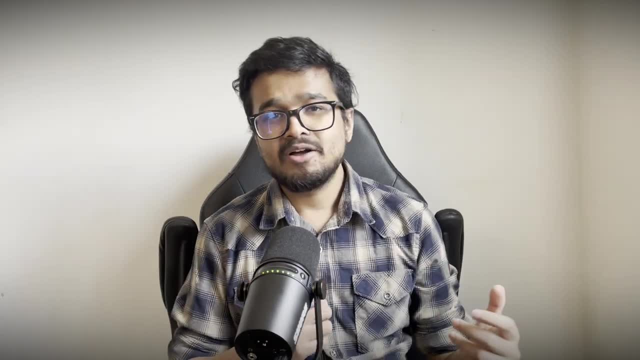 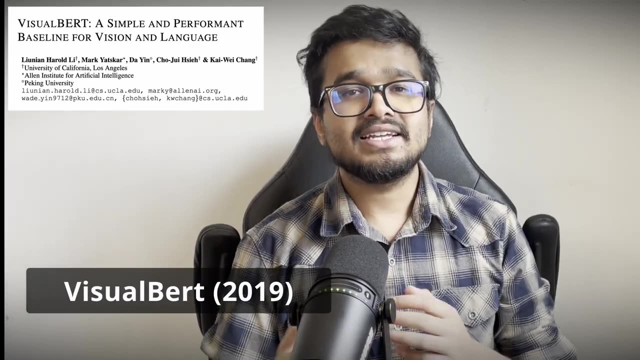 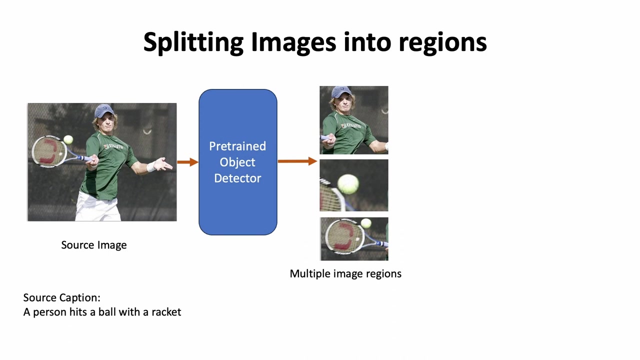 learning is great when it comes to aligning paired data, but another method to align multimodal datasets is masked visual language modeling in visual bird. instead of using entire images as input to the model, the author's first split up the image into multiple regions using a pre-trained object detector. this 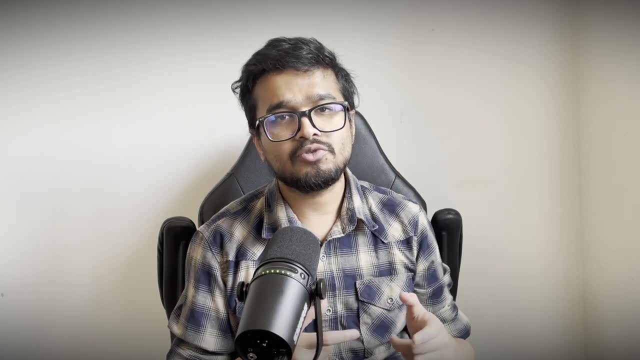 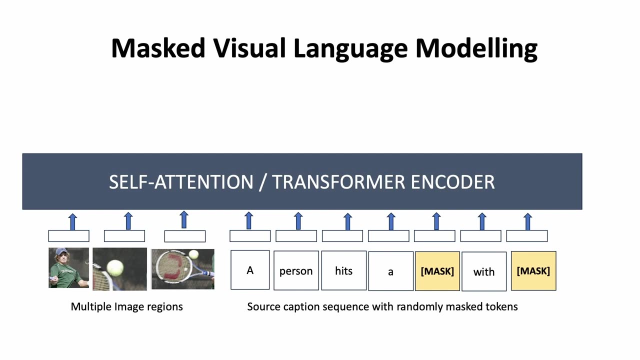 sequence of region embeddings is passed into a transformer self-attention model along with the images description, but random tokens from the text section is masked or replaced randomly. the network then has to process this entire input to guess what the masked description tokens were. this process of perturbing the 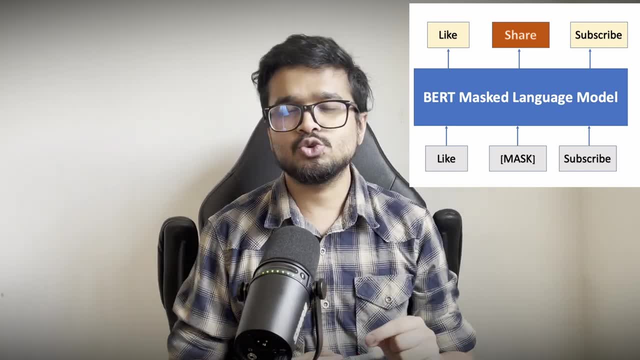 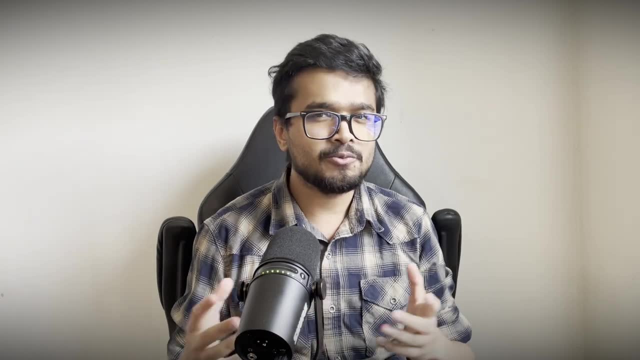 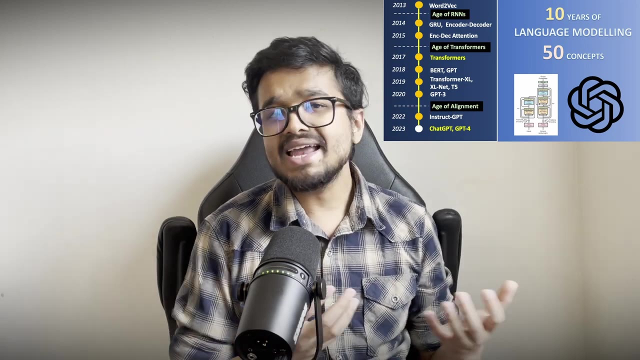 input sequence with marks, tokens and training the neural network to reconstruct the original input is called masked language modeling. if you're unfamiliar with how transformers or BERT or attention work, feel free to check out my previous video where I cover these topics in more depth at a high level. the self-attention layer. 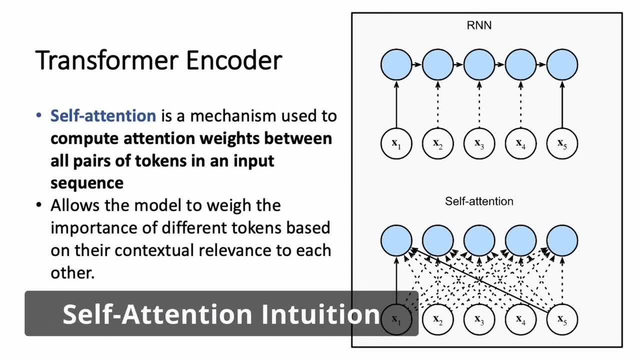 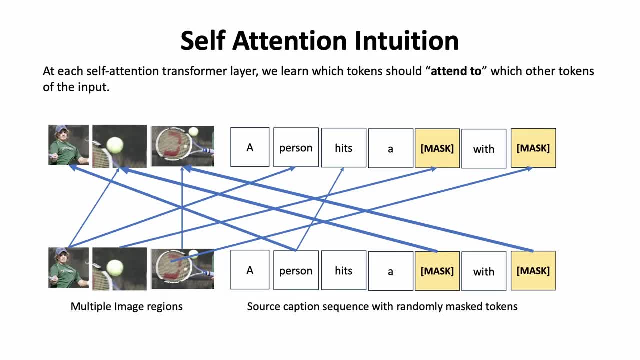 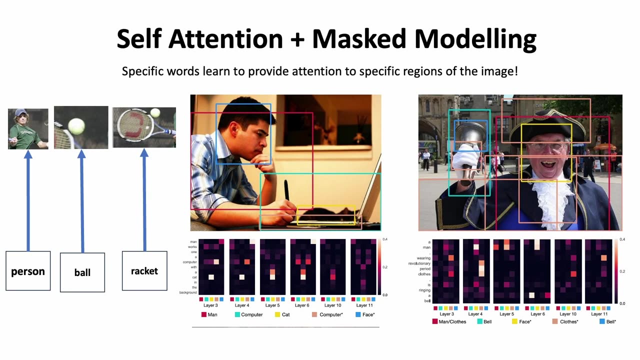 in the encoder holistically processes the entire sequence of image, region embeddings and text description embeddings, by contextualizing each of the tokens in the sequence with each other, such that each token- visual or text- learns which other tokens to provide the maximum attention to. also, by splitting the image into specific regions, we also learned the dependencies. 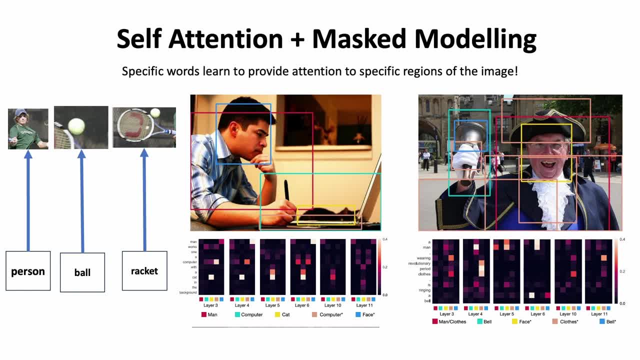 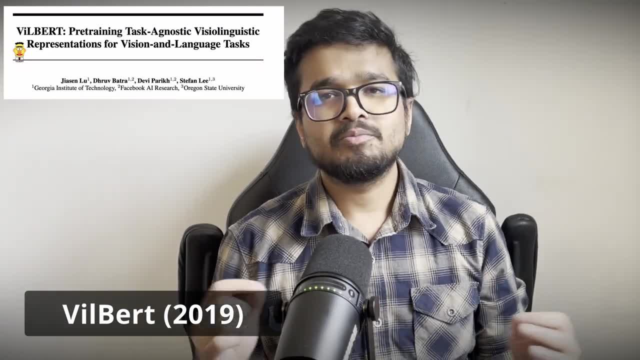 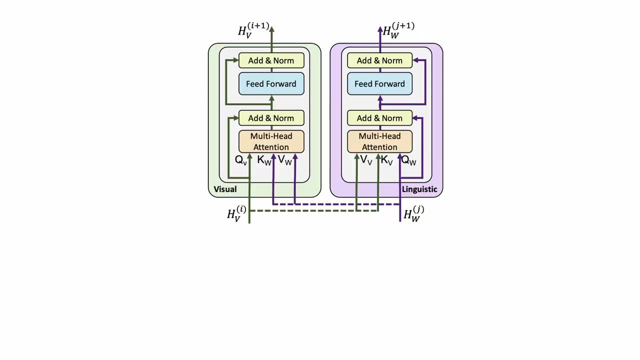 of specific text tokens in the descriptions, with specific regions that appear in the image. a concurrent paper called Vilbert also uses masked language modeling, but they train two separate self-attention transformer encoders, one for the image, the other for the text. after each self-attention layer they 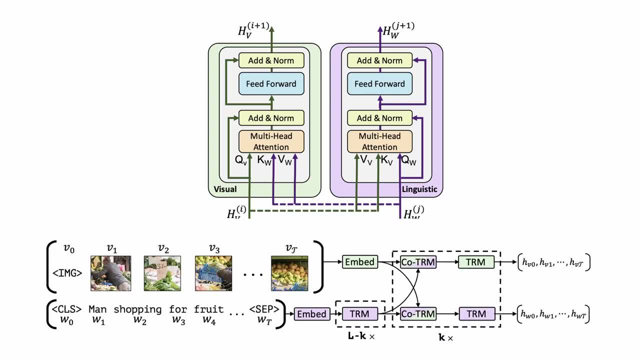 include a code attention layer where the embeddings of each modality learns to attend to the embeddings of the object. so we will be talking aboutrating pornography layer. so, after the capacitival practice of coding a math model, we will also добавl embeddings of the other modality, exchanging information between the two. 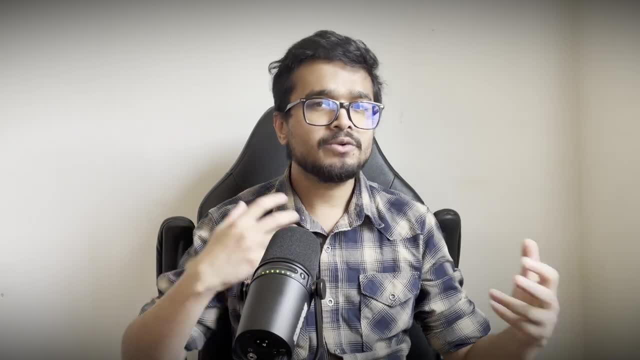 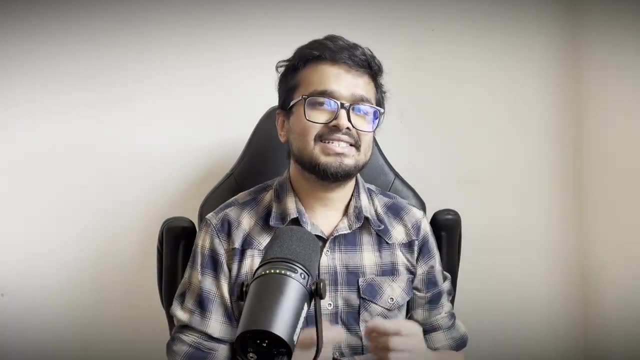 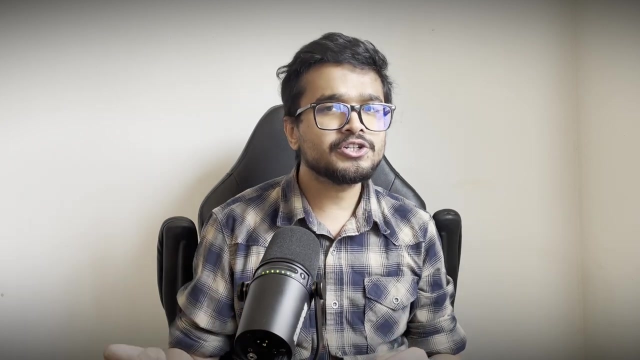 modalities at each transformer layer and learn more and more complex dependencies with each layer. Both Wilbert and Visualbert are excellent pre-training techniques that can learn image and text representation from volumes of data. These learned embeddings can then be used for further downstream tasks by 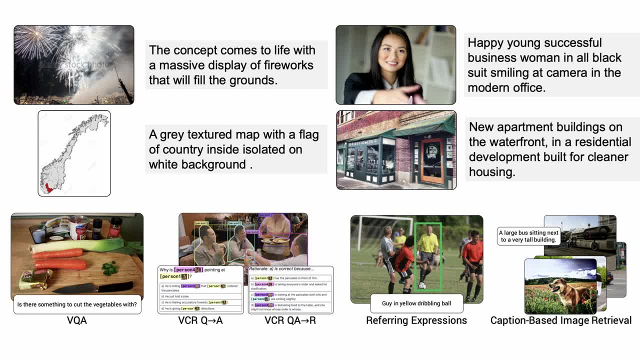 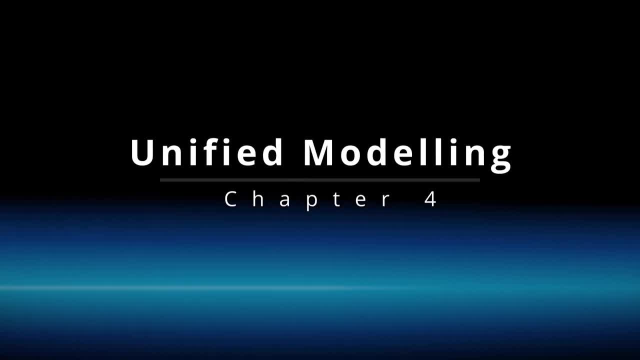 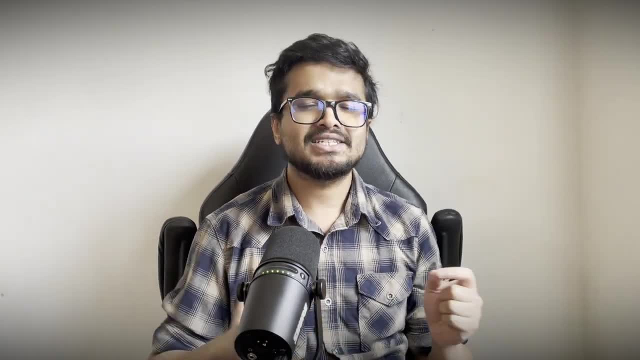 fine-tuning them on specific datasets and tasks, such as captioning, visual question answering, image-text matching and more. So far we have talked about discriminative modeling that tries to align multimodal input by training them on a single task, such as contrastive learning or masked modeling. But training 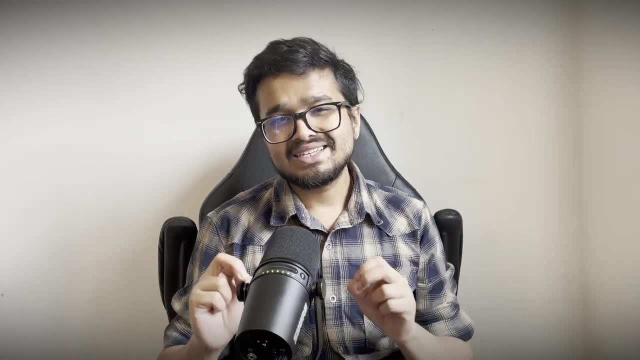 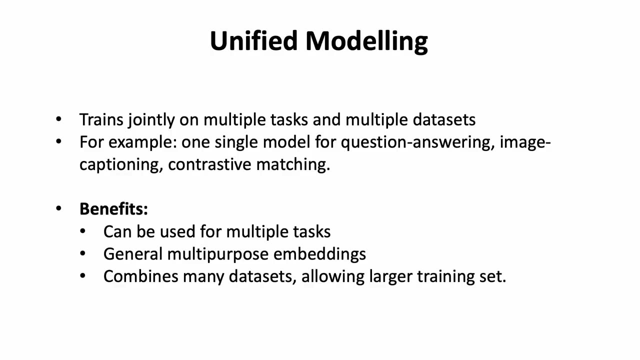 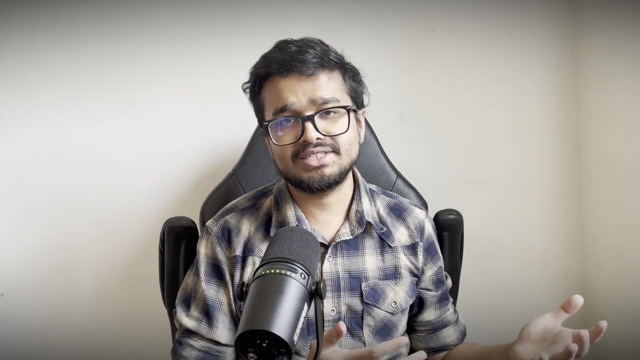 on a specific task, like question answering or captioning, still requires fine-tuning these models with a separate network. In contrast, unified modeling aims to combine multiple datasets together and train a single model on diverse tasks like image captioning, mask filling, visual question answering and more. This makes the model learn generalized. 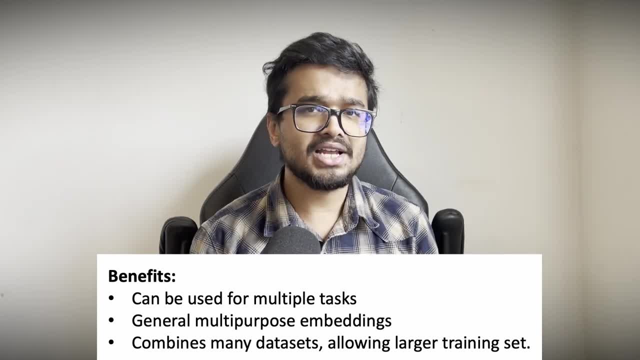 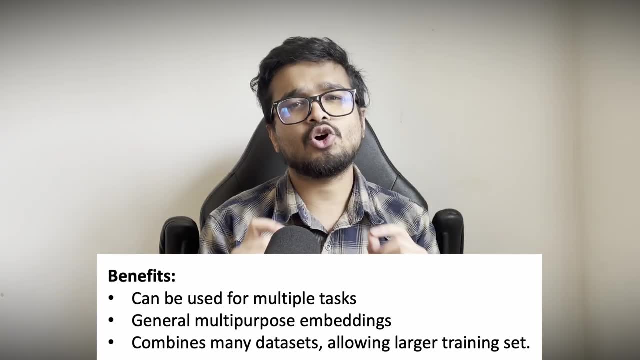 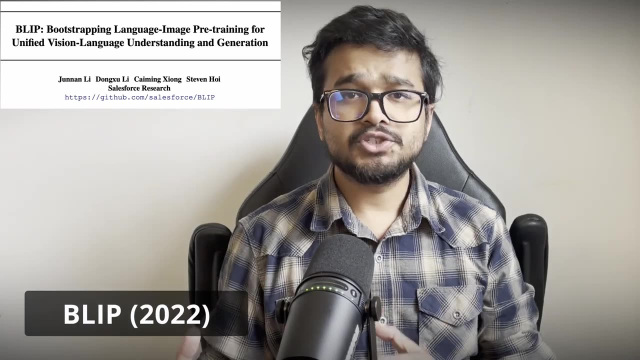 embeddings that can be used for a wide range of downstream tasks, and also combining multiple data sets together makes the total training data much larger than any single contributing dataset could have made. The B Rule Model trains a unified model that jointly optimizes on three objectives. First, a 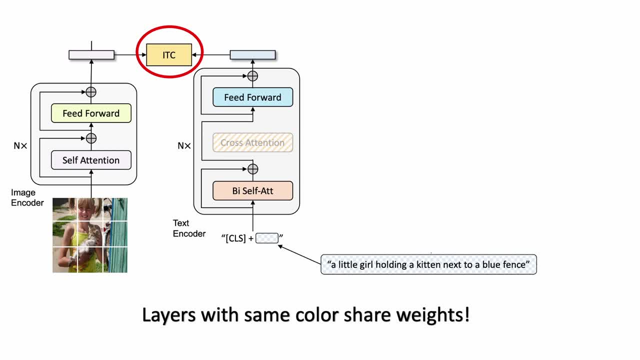 contrastive loss, where the image and text embeddings are processed independently, like CLIP. Second, an image-text matching task, where the text embeddings are processed with self-attention and the image embeddings are used as cross-attention to do binary prediction whether the input image 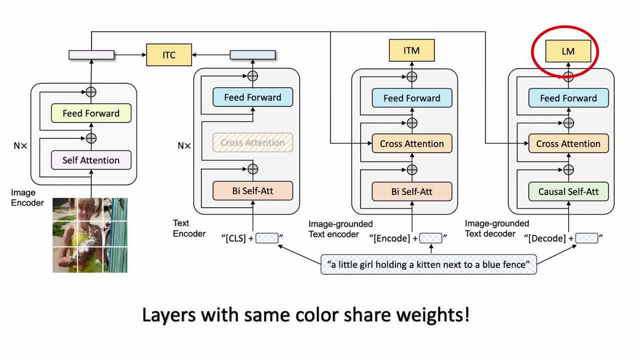 and text are a positive pair. Thirdly, an autoregressive language model is trained, combining causal mass attention on the text and cross-modal attention with the image to generate captions, token by token. Notice that these three models share the same layer weights across each architecture, so 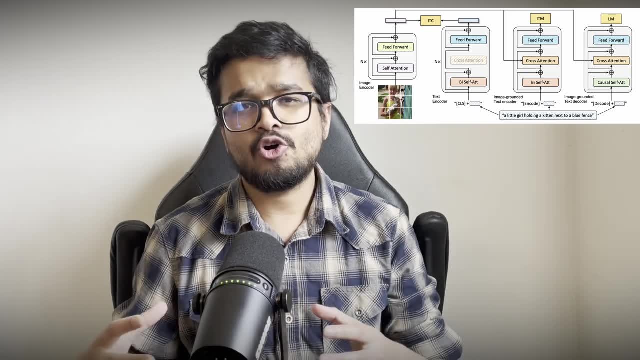 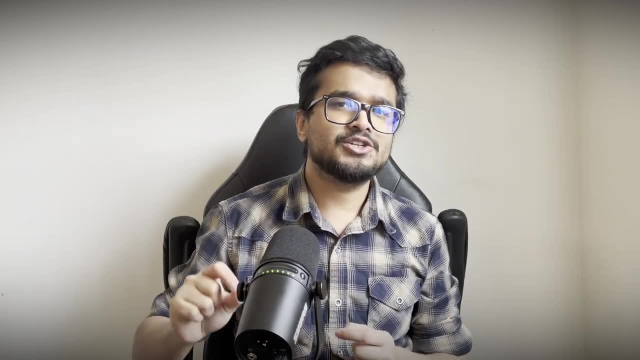 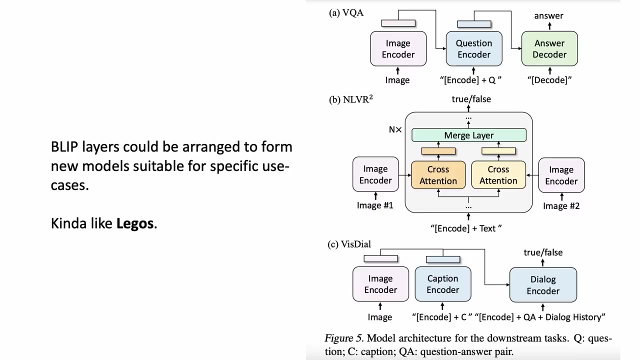 these weights are trained to be generalizable and applicable for all three tasks. Blip achieves some great metrics on the three tasks it was trained on, but we can also transfer learn to other downstream tasks, like visual question answering and visual dialogue, by using these pre-trained weights and adding small layers on top to fulfill the target. 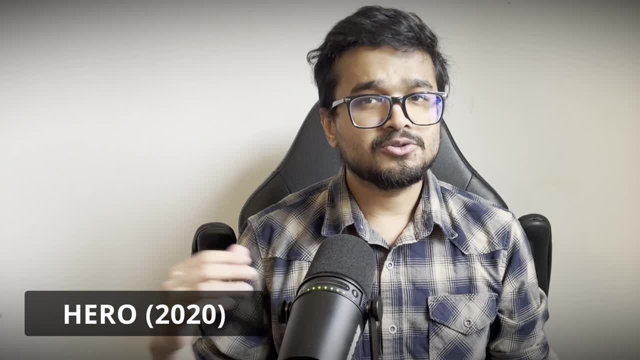 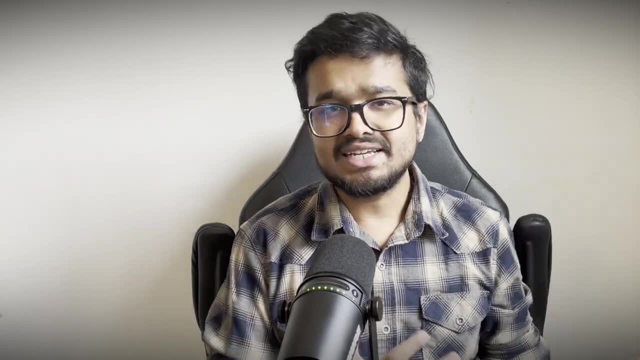 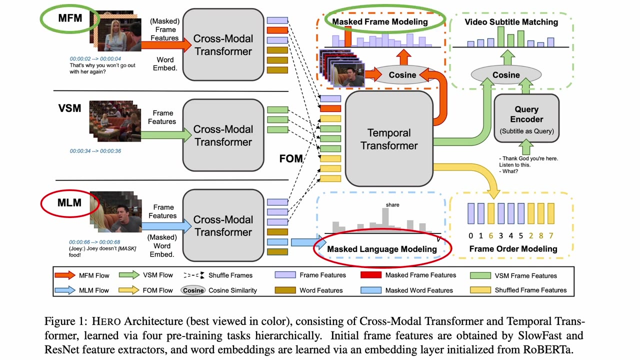 task. Another example that follows a similar multi-task objective is the hero pivot. They work with a dataset containing videos and their subtitles and train an attention-based model on multiple tasks like mask language modeling from text, mask-free modeling, where we output the most relevant frame from the video given an input: word frame-order matching. 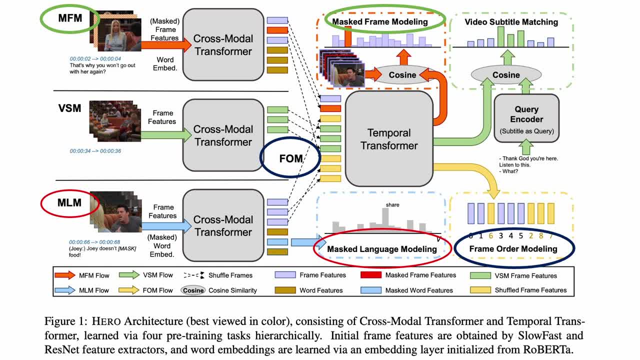 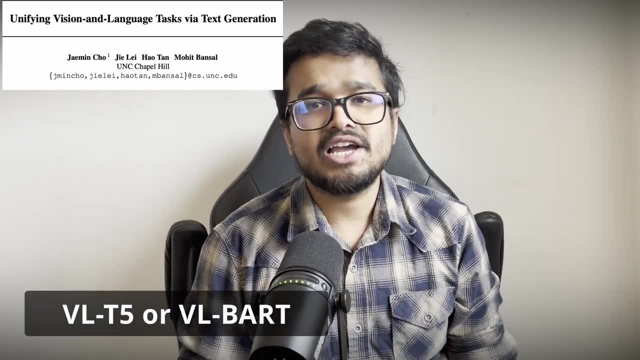 which inputs frames from a video in random order and arranges them correctly. and video subtitle matching, which inputs a subtitle prompt and provides a likelihood of the video being recorded. Another model that has a slightly different take is the VLT5 or VL-BART model, which converts 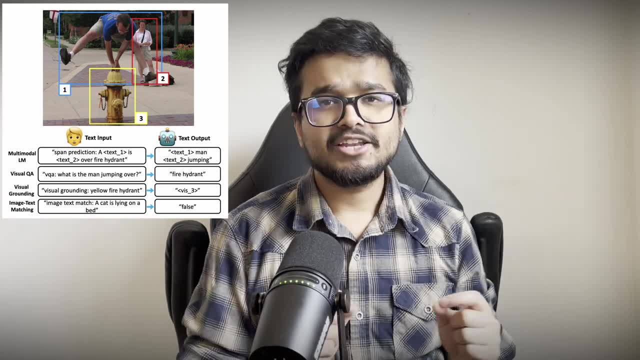 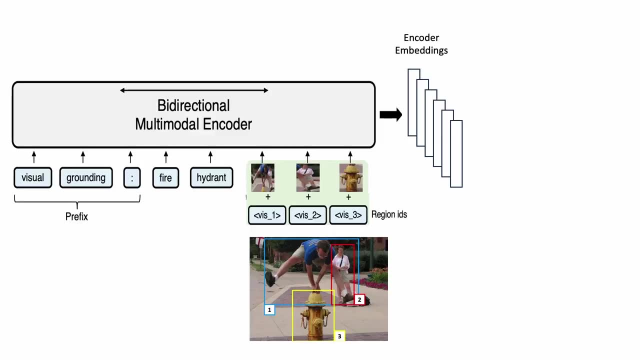 multiple tasks into a sequence-to-text task and uses a transformer encoder-decoder architecture to generate natural language outputs. The encoder inputs, the representations of multiple regions of the image obtained through an object detector and special region ID tokens, along with a sequence of text prompt tokens. 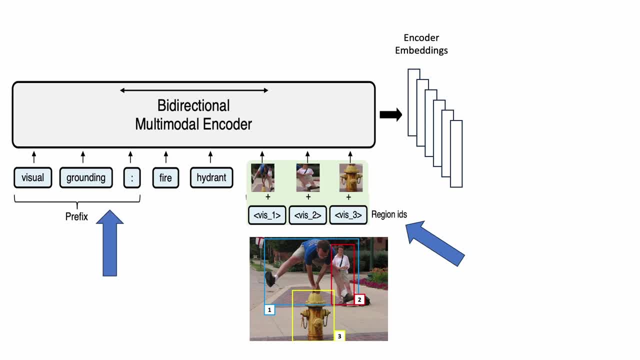 The encoder inputs, the representations of multiple regions of the image obtained through an object detector and special region ID tokens, along with a sequence of text prompt tokens. The encoder inputs, the representations of multiple regions of the image obtained through an object detector and special region ID tokens, along with a sequence of text prompt tokens. 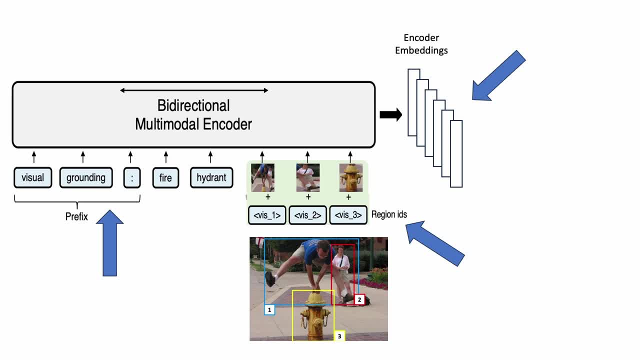 It then encodes this entire input into a joint sequence of embeddings. using self-attention, The decoder then applies attention to the encoder sequence and autoregressively generates the response, one token at a time. A technique like this allows us to generate captions with free-form text and even allows 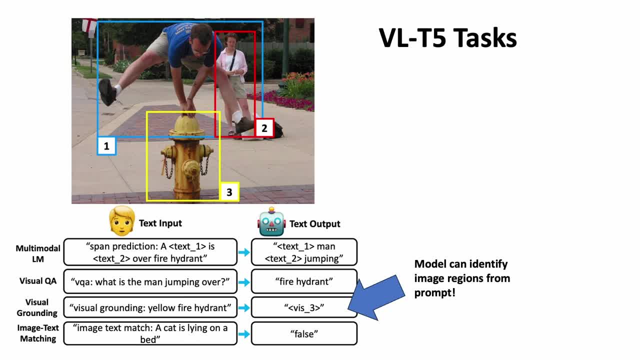 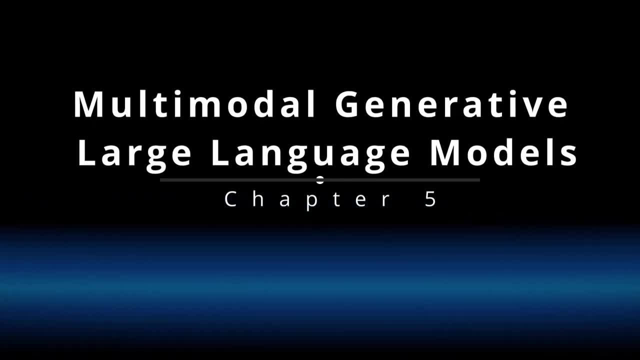 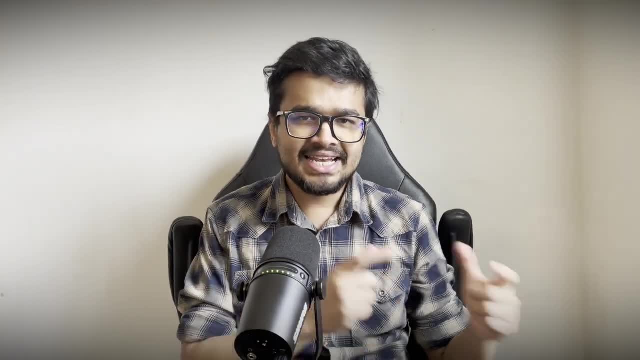 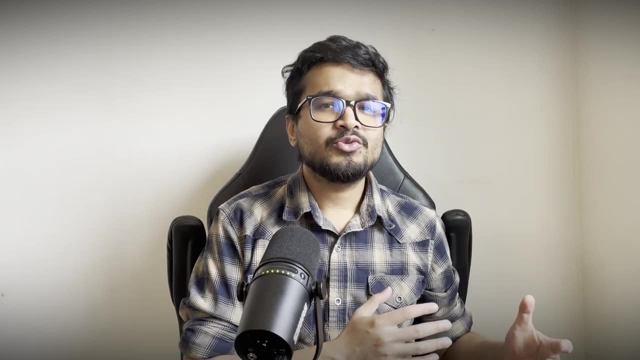 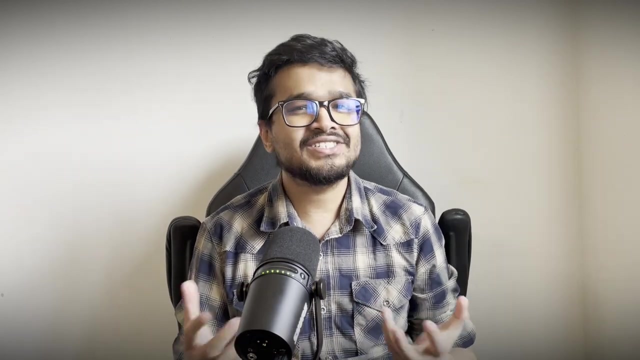 What is VLT5?? So far, the models we have discussed have mostly been training the text and image encoders from scratch. However, the early 2020s to 2021 was an era where we were moving towards large scale generative language models like GPT-2 that were trained on gigabytes of text data. 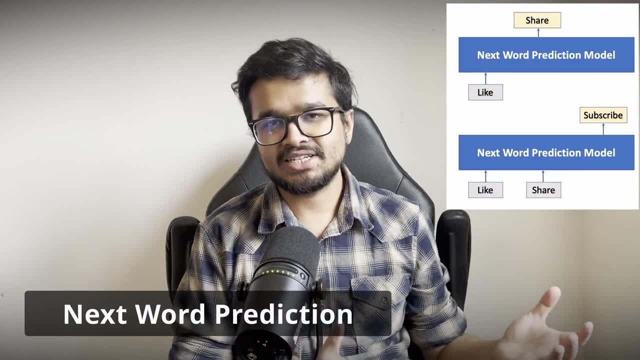 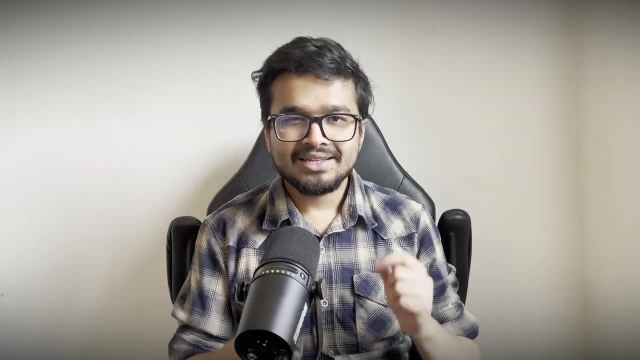 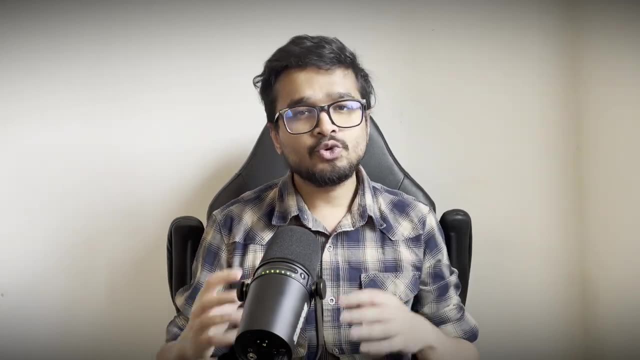 Basically, these models were trained on next word prediction tasks, meaning they were able to generate the likelihood of the next word given a sequence of prefixed words. These models were demonstrated to have encyclopedic knowledge by learning to model natural language and generate fluent text when prompted correctly. 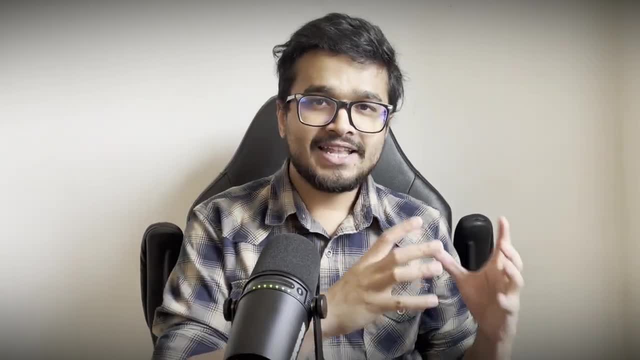 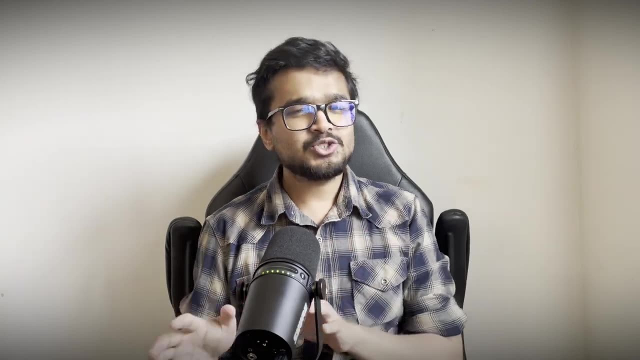 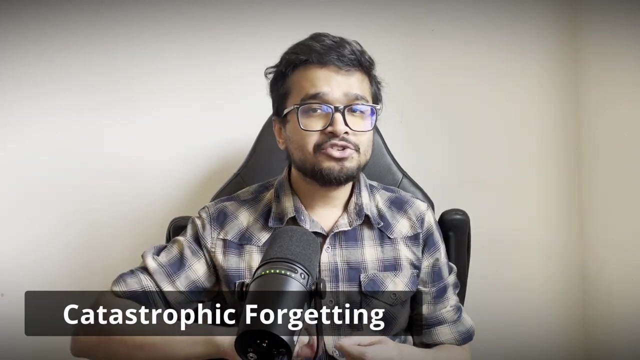 Wouldn't it be really cool if we could transfer all that knowledge of a generative text model into a multimodal setting? That sounds enticing on paper, but it actually imposes some tricky practical challenges. For example, taking an LLM that has already been pre-trained on gigabytes of text and 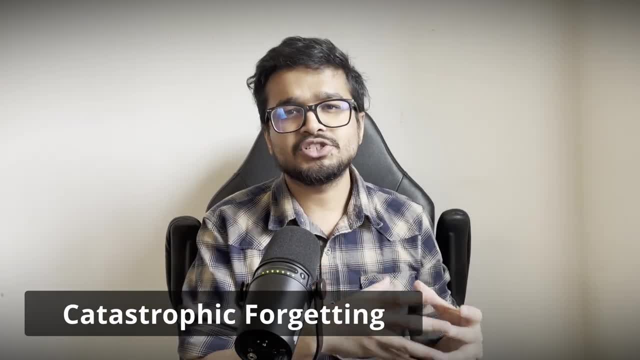 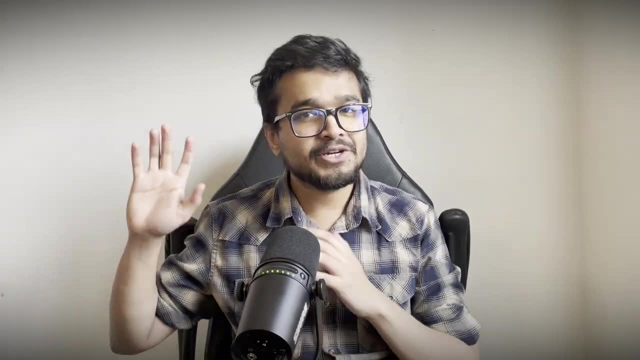 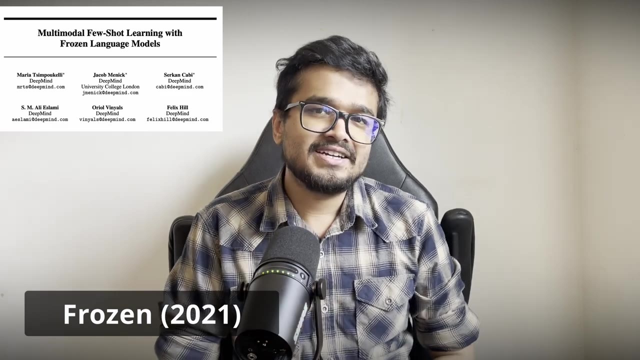 then fine-tuning it on a smaller, noisy image captions dataset can lead to something called catastrophic forgetting, where the LLM just forgets things it has learned during pre-training in favor of over-optimizing its weights to the current task In 2021, the Frozen paper addressed this LLM fine-tuning problem by freezing the weights. 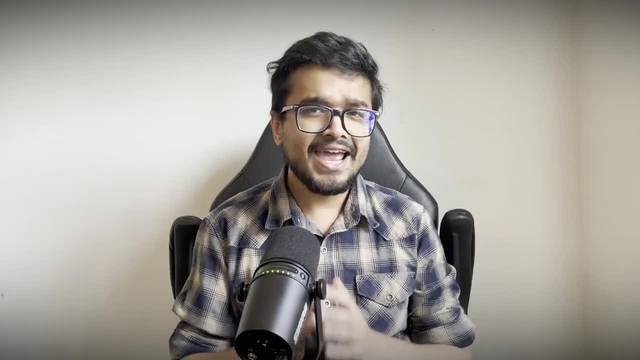 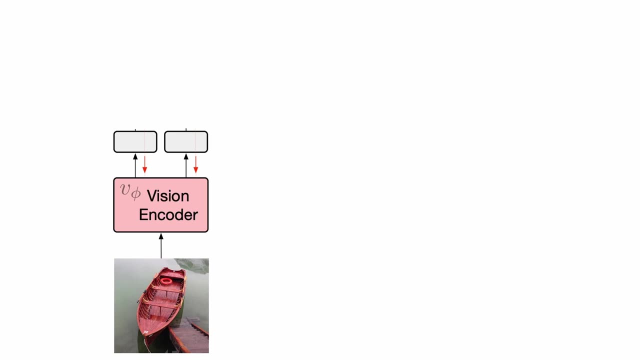 of a pre-trained 7 billion-parameter generative LLM and only training the vision encoder. A ResNet encodes the image. The image is rearranged to form a sequence of embeddings, each having the same dimensions as the token embeddings of the pre-trained LLM. 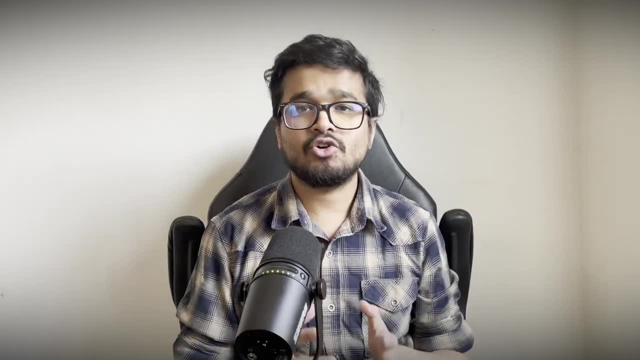 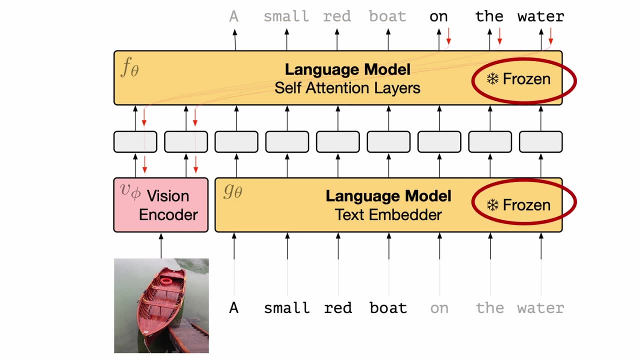 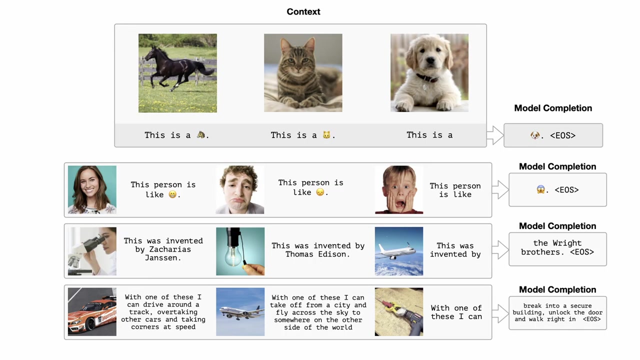 This sequence of embeddings is inputted into the LLM as a prefix or visual prefix and the image caption is generated one token at a time. Since the LLM weights are frozen, the gradients only update the weights of the vision encoder Frozen showed some really cool zero-shot transfer to multiple tasks on unseen data, like identifying. 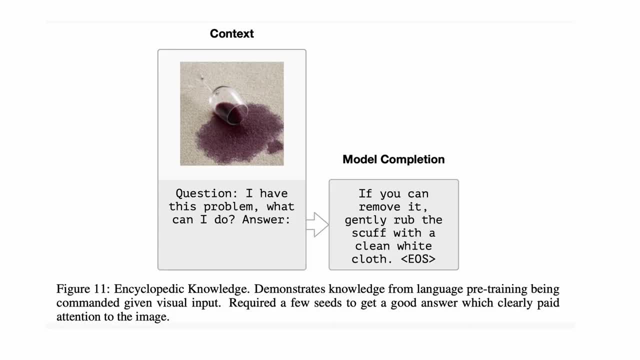 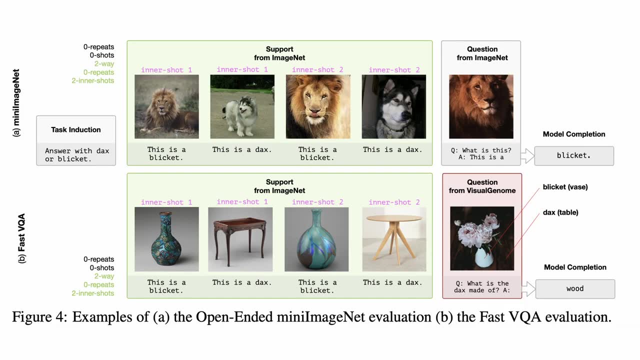 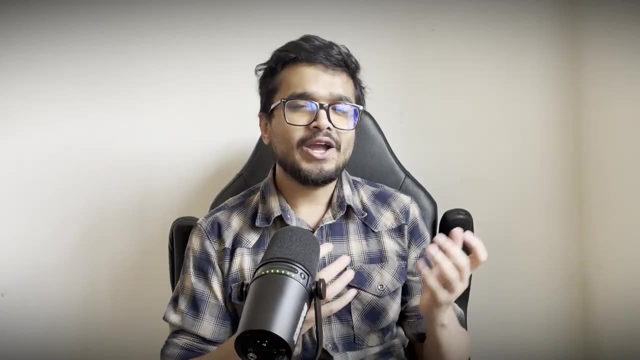 objects or answering questions about images. They also showed some few shorter abilities, where they pass random names of images into the model as prompts and the model is able to categorize the new images accordingly by looking at the inputted prompt. Of course, if you can use pre-trained LLMs, why not also use pre-trained vision encoders? 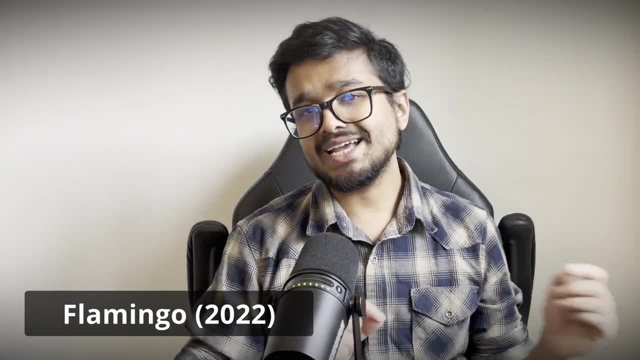 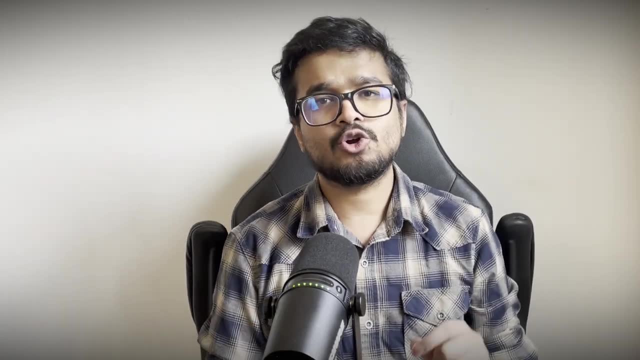 as well. That's what the Flamingo paper does. Their text encoder is a pre-trained LLM trained on next-word prediction, and their vision encoder is a ResNet model Pre-trained on good ol' contrastive loss on an image-text-captions dataset. 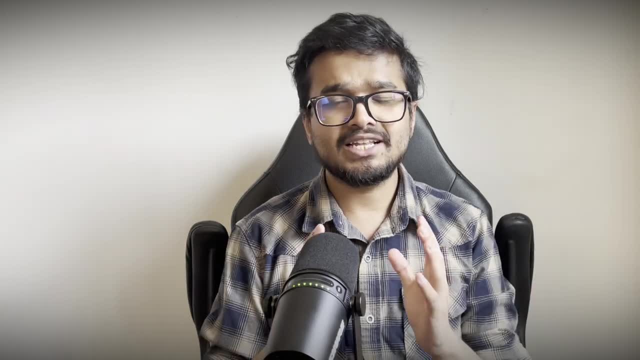 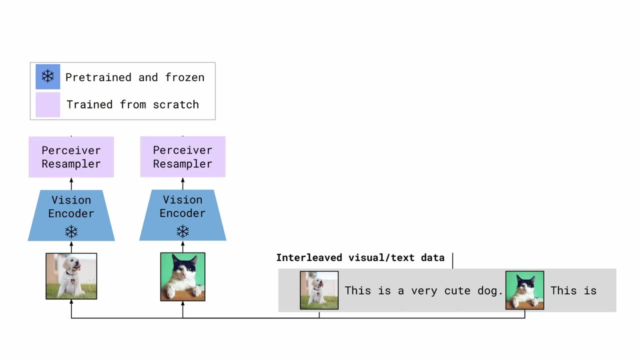 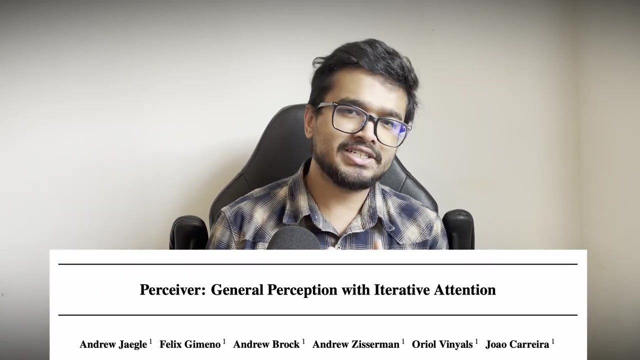 To align these two independent pre-trained models into a single multimodal model. they do the following: The vision encoder output is passed into a Perceiver network which maps the image or video embeddings into a fixed sequence of embeddings. Perceiver networks are neural networks that uses cross-attention mechanism to efficiently. 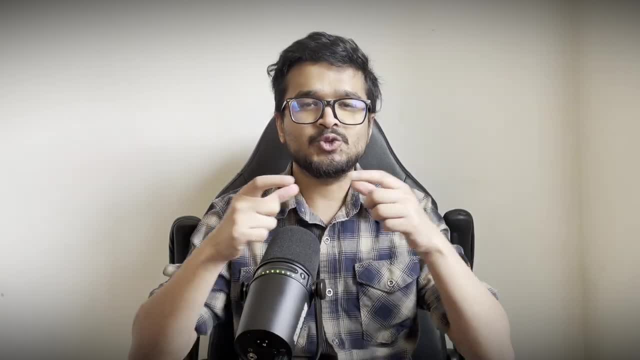 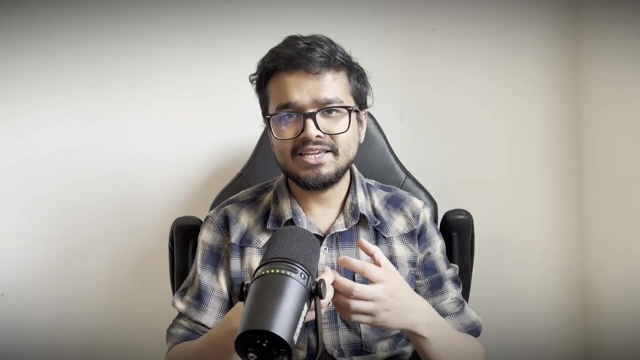 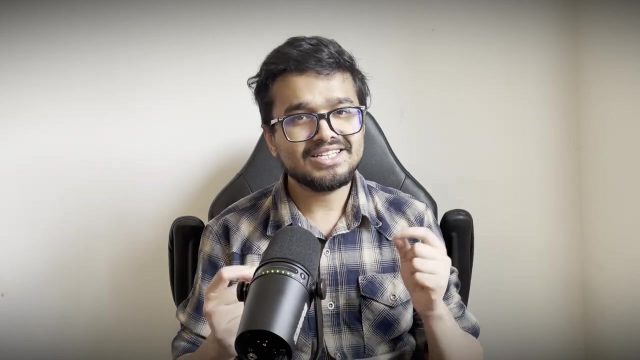 map inputs of arbitrary sequence length into a fixed sequence length. This compresses the number of tokens reserved for visual embeddings and compresses the input to its essential content, making the size of the embeddings independent of the image or video resolution. This allows Flamingo to input high-resolution visual inputs that will otherwise be impossible. 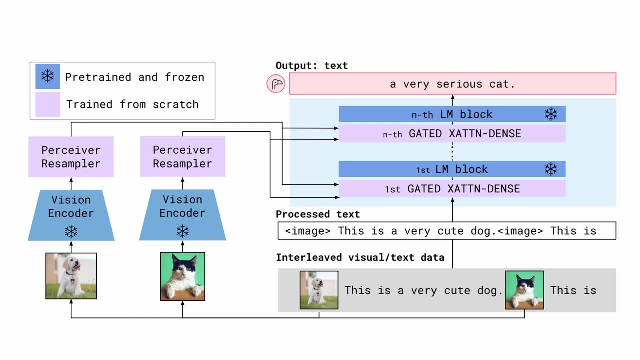 For the LLM model 2, each transformer layer is kept frozen and new trainable gated cross-attention layers are introduced between each layer. that conditions the language model on the visual embeddings. This approach is very useful for the LLM model 2.. 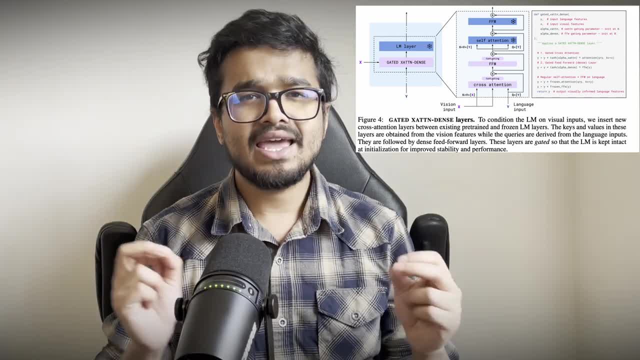 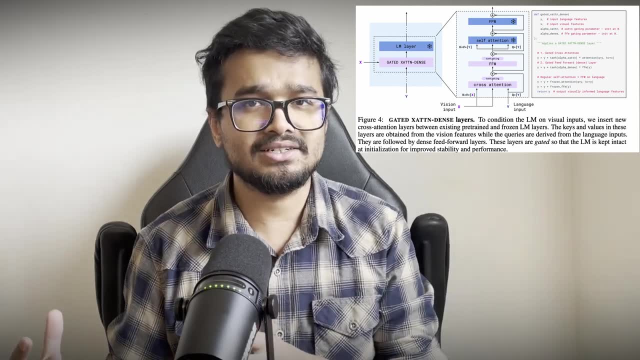 This approach is pretty cool because it does not try to update any of the learned LLM weights, but instead adds new weights in between each transformer layers to add information about the visual content. While training, the network only updates these image Perceiver layers and the cross-attention. 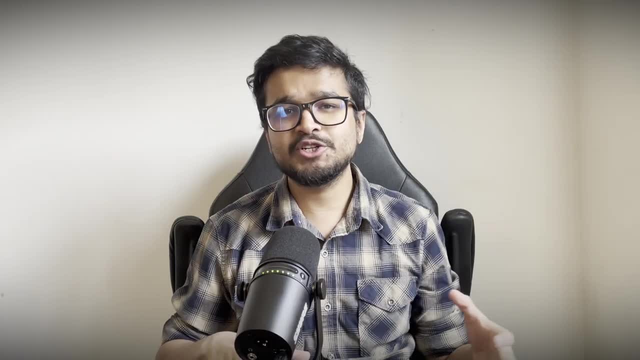 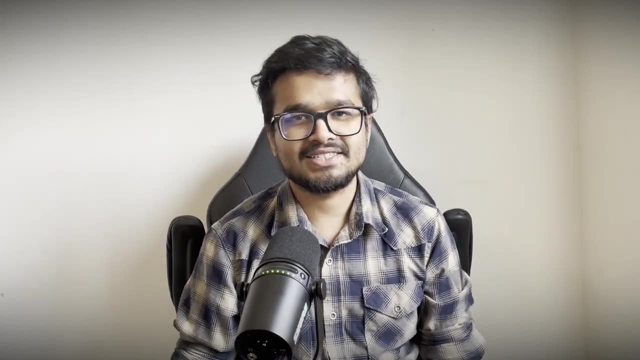 layers to align these two universes together without needing to throw away the pre-trained weights. Smart right Flamingo shows some truly crazy results on zero-shot tasks like captioning images, answering questions about multiple images. This approach is pretty cool because it does not try to update any of the learned LLM weights. 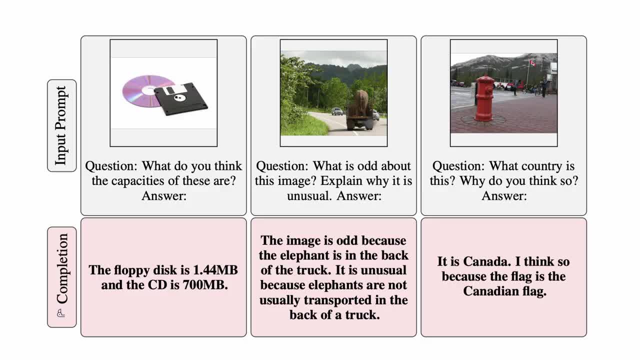 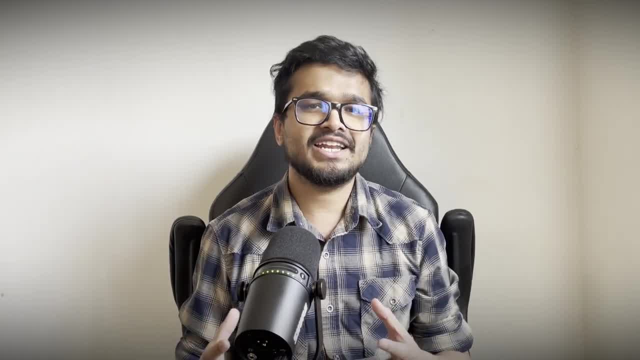 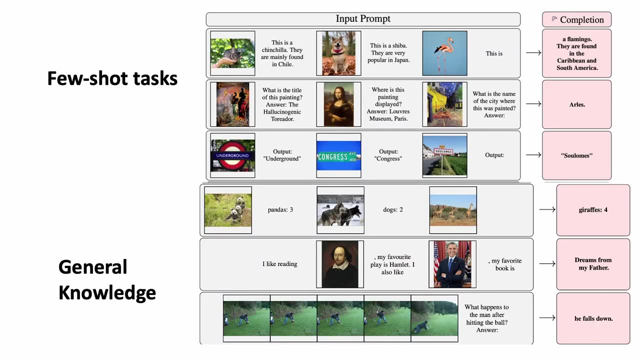 describing actions from videos, all in zero-shot. But what is even crazier are the few-shot tasks. The encyclopedic knowledge of LLMs as well as the image understanding of the pre-trained vision encoders are very evident. For example, prompting the model with images to read signboards, answering general knowledge. 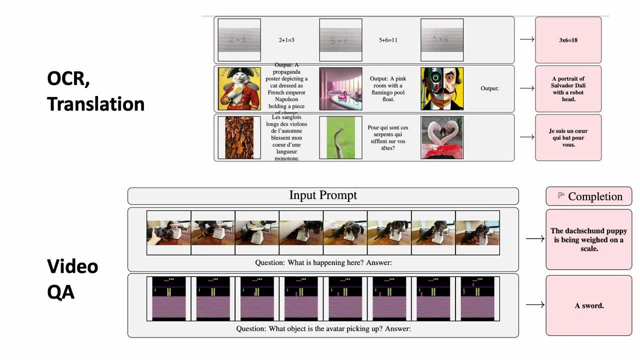 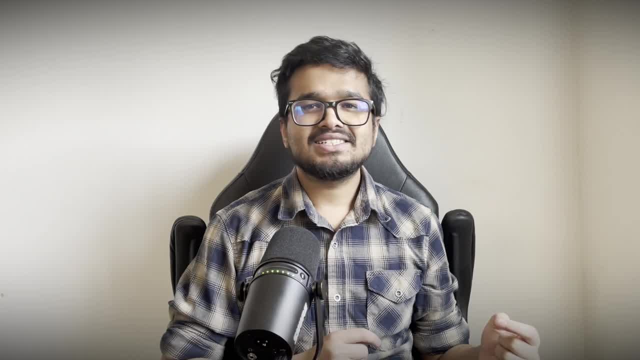 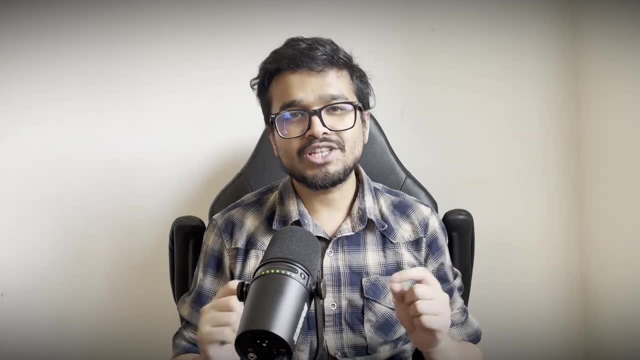 questions predicting the future of a video sequence, responding in a foreign language and engaging in visual dialogue shows the power of few-shot learning. We can pass in examples to the model at inference time and it gets conditioned to output in the same format to new inputs without ever needing to fine-tune or retrain the model. 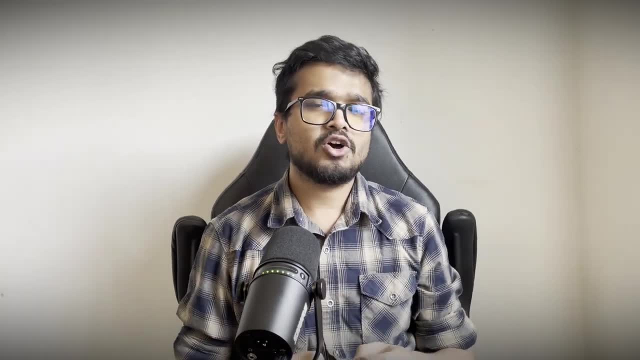 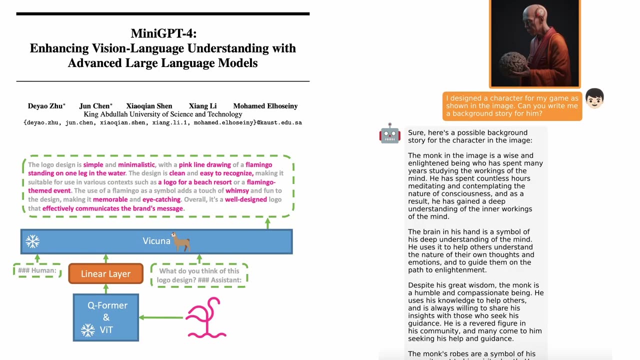 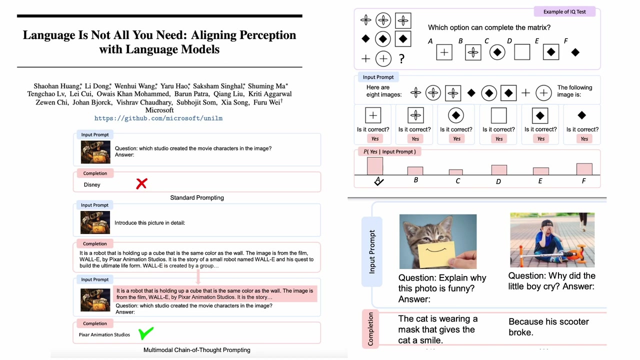 on those specific use cases. A similar approach is adopted by MiniGPT-4, which inputs the embeddings of a pre-trained vision encoder through a simple linear layer into a pre-trained LLM, While Cosmos 1 from Microsoft is also able to do a bunch of cool stuff like IQ tests. 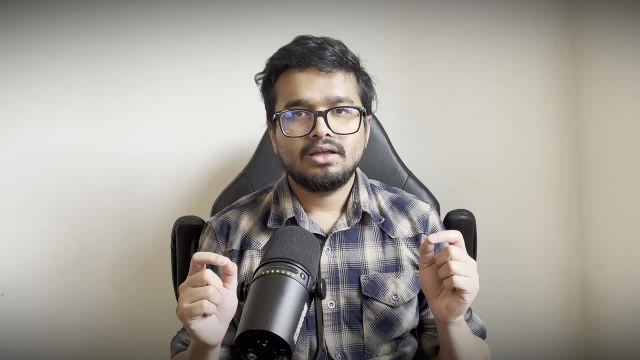 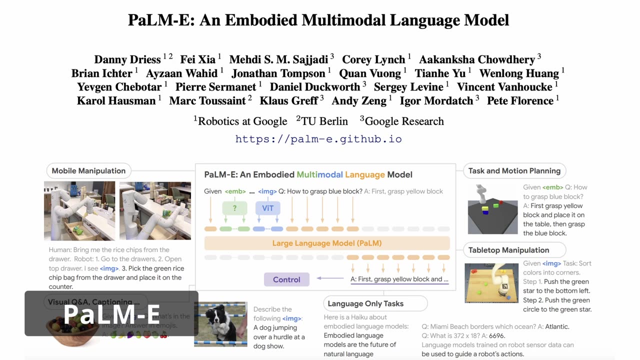 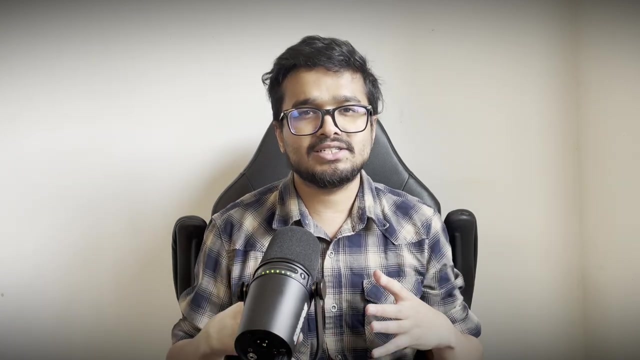 explaining jokes from images and chain of thought. question answering. The Palm E model by Google uses their text-only large language model called Palm to train Embodied Model for robotics use cases. Embodied language models are a type of model that also learns the physical presence of. 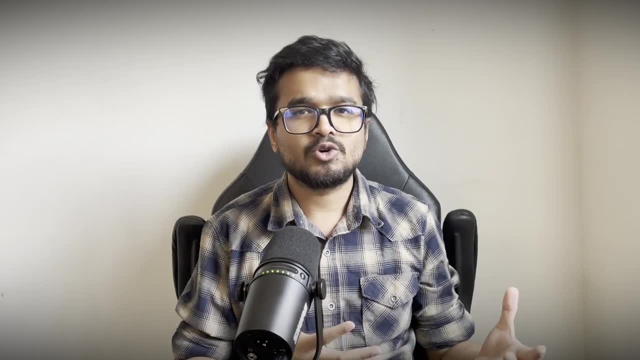 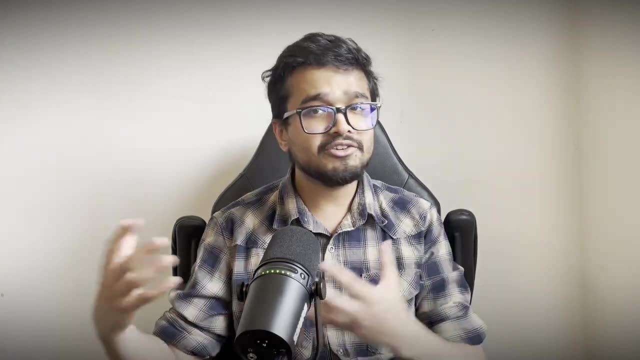 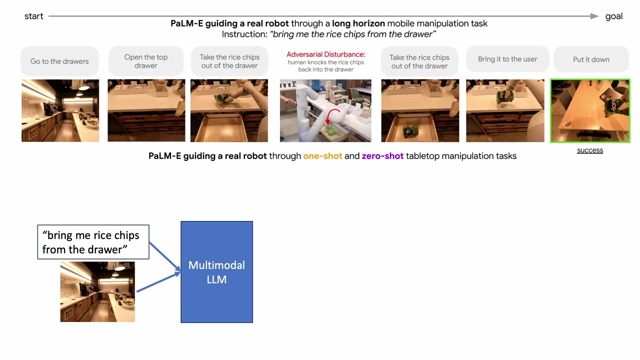 the AI alongside language. This means that the multimodalities explored in Palm E extend beyond images and text, but also state vectors of the robots or its environments, like size, size of the robot, size of the robot, etc. For performing the robotics planning and tasks, they provide the relevant multimodal prompt.